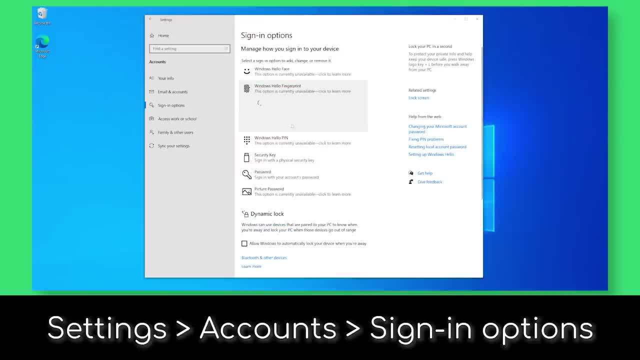 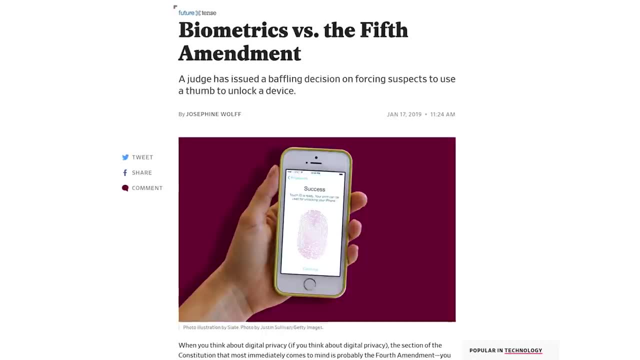 Once you set a strong password, you may then have the option to utilize biometrics. These typically suffer three problems. One, they can be cracked fairly easily. Two, they fall under different legal jurisdictions in some countries, meaning you can be forced to. 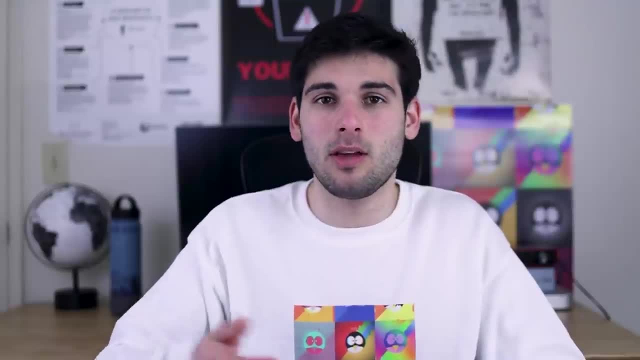 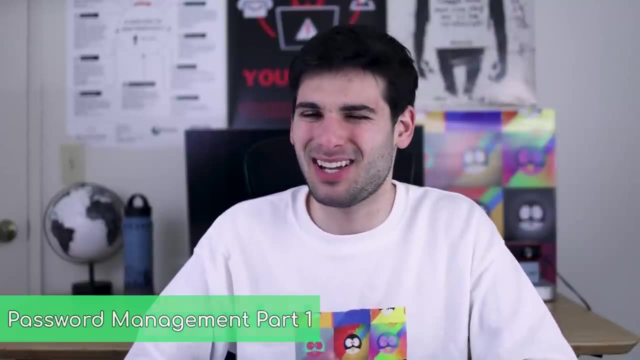 unlock your device if it's utilizing biometrics. And three, some users have privacy concerns behind biometric data stored on their devices. Passwords you use on websites are a commonly left out part of your security If you use the same or similar password for all of your services. 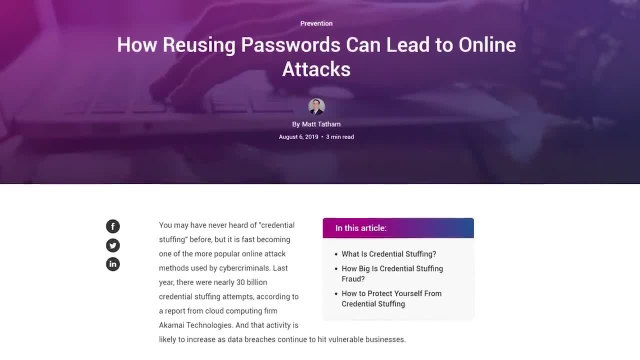 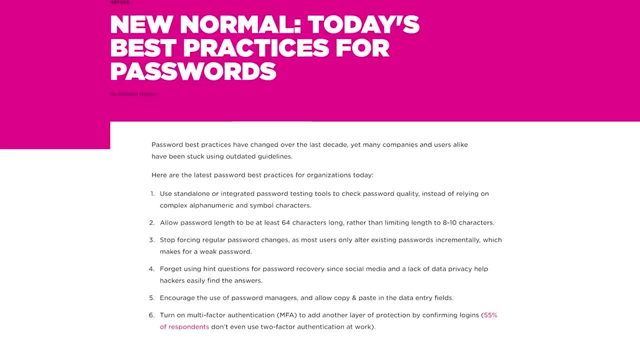 one breach can very easily lead to the others being breached since they utilize the same or similar credentials. Make sure- at least in Zone 1, that you are using strong, unique passwords. I'll leave a source on what that means and different methods of doing it. Zone 2 will go. 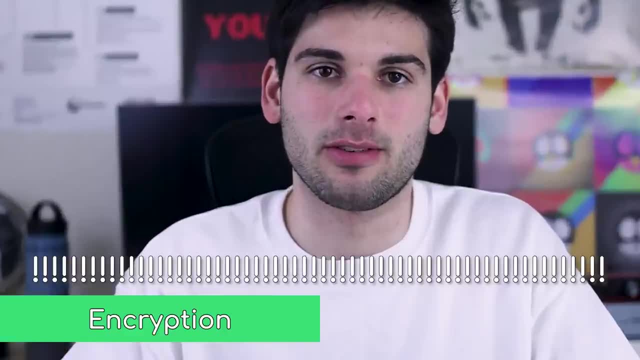 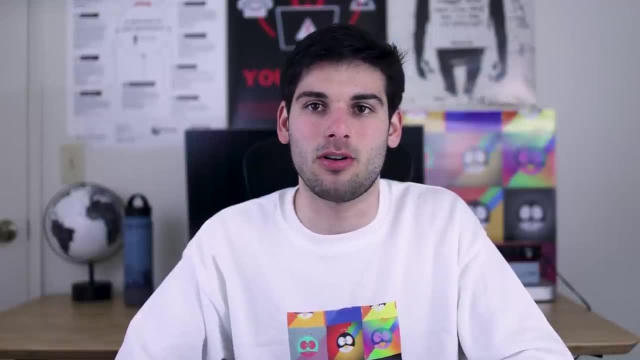 further into this. By default, Windows does not encrypt your files. It's kind of crazy. Even with a Windows login password, anyone can gain access to your files in just a few minutes with little to no technical knowledge. I don't know why no one talks about this. Watch our video demoing how this 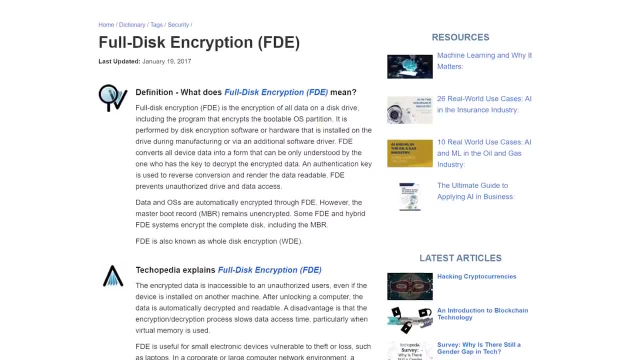 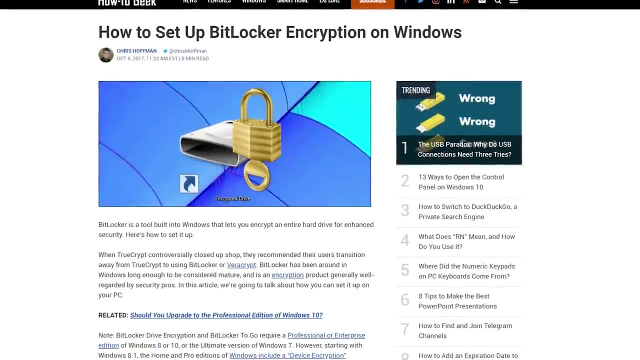 is done To prevent this. use full disk encryption. It should be a staple. Windows has BitLocker built pro version because security is paywalled by Microsoft for some reason. So if you're on pro or higher, just go into your settings and enable BitLocker If you're someone who doesn't pay for. 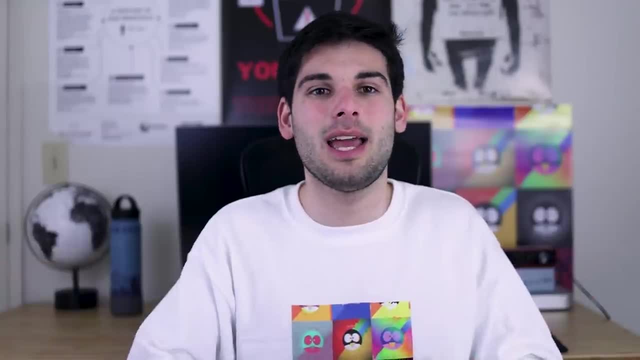 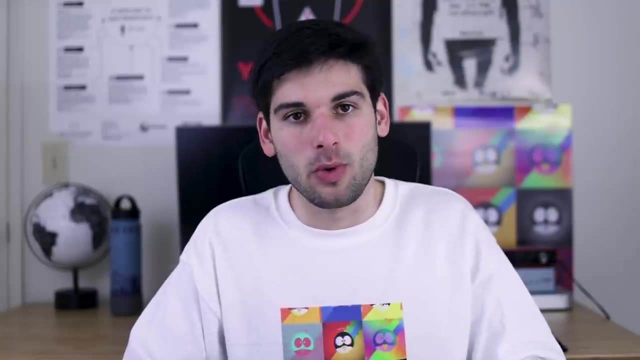 their operating system, aka Windows home users. we recommend really any form of full disk encryption, though our top recommendation is VeriCrypt, a great free and open source tool. However, we also believe proprietary full disk encryption is still better than no full disk encryption. So 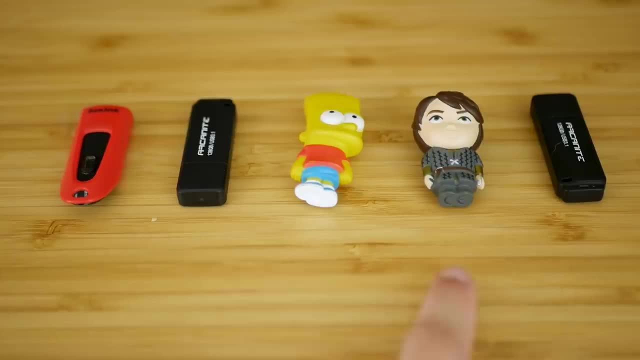 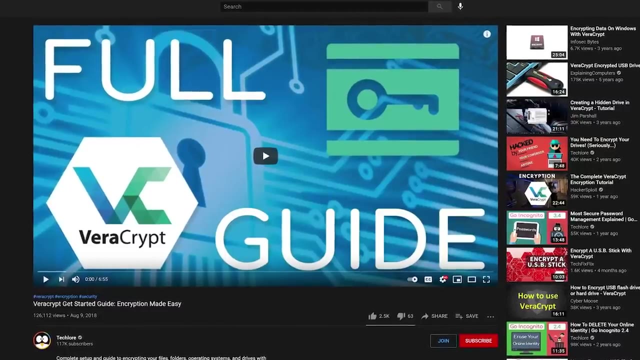 feel free to explore different options. Similarly, if you have any external USBs or external drives backing up your data, we encourage you to use VeriCrypt on those devices as well. We have an in-depth guide covering how to use this tool to make it easy to understand for everybody. 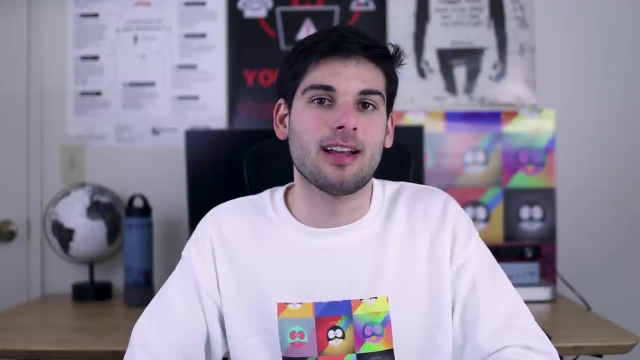 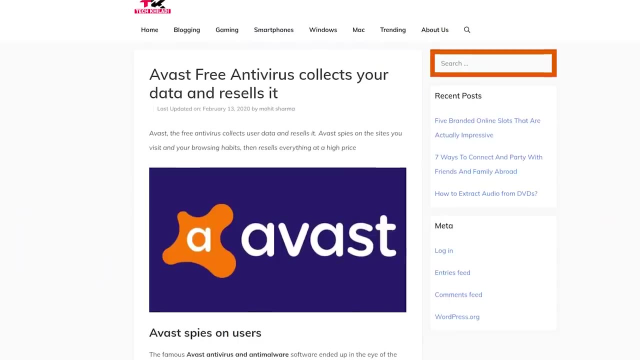 Antiviruses are tricky, as they can improve security, with often a detrimental impact to your privacy, as they pretty transparently tell you how much of this data they collect. The first thing everyone should do is stop using their free antivirus from a commercial company. 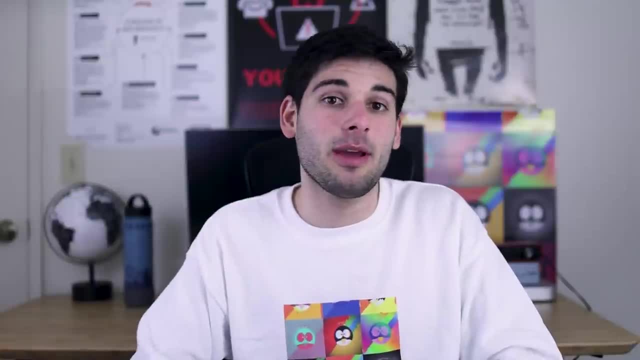 with no business model, Just don't Up. next, we recommend most people just stick with Windows Defender. It's free, it's effective and it's frequently used. So if you're looking for a free version of Windows Defender, this is the one for you. Windows already collects a lot of. 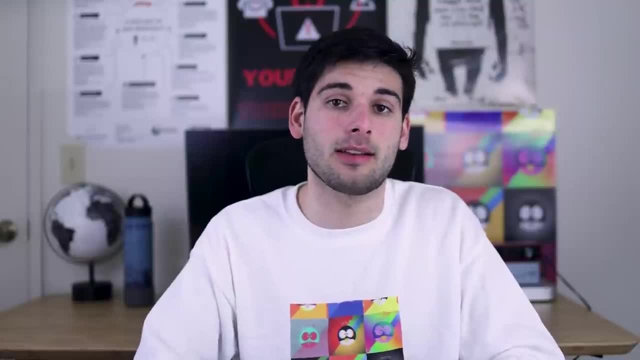 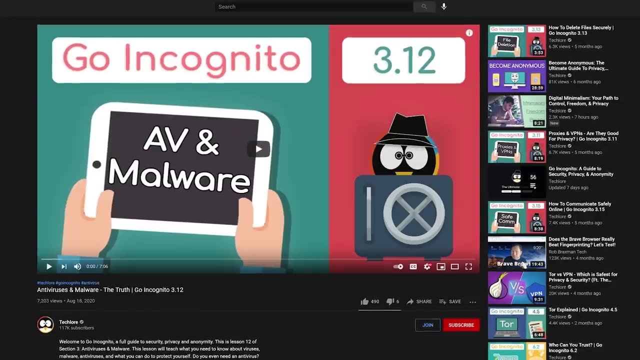 your information, so at least this way you can prevent two companies from getting access to it. There are a few exceptions for people who may want a paid solution, though not many fall into that boat. We have a Go Incognito lesson that dives deeper into this For most of you watching. 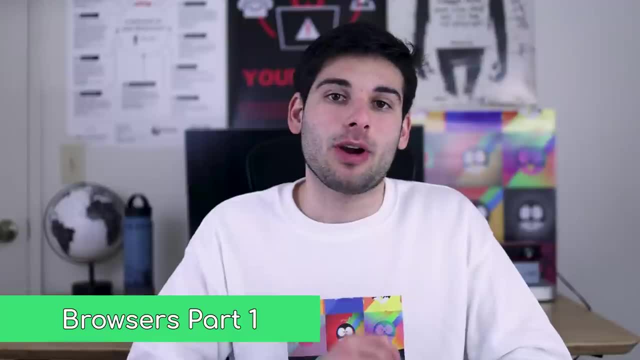 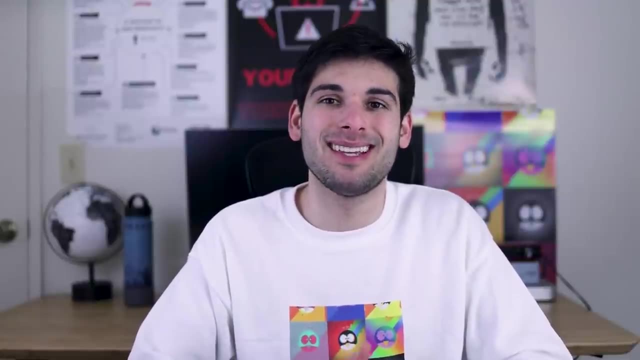 Windows Defender is definitely the way that we want to push most of you. Your browser has the ability to track everywhere you go on the internet. Ensuring you are using something with proven security and privacy is paramount to protecting your web traffic. The newest version of Windows Defender is the latest version of Windows Defender. 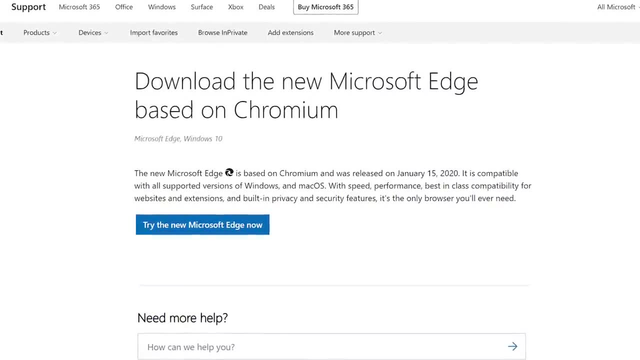 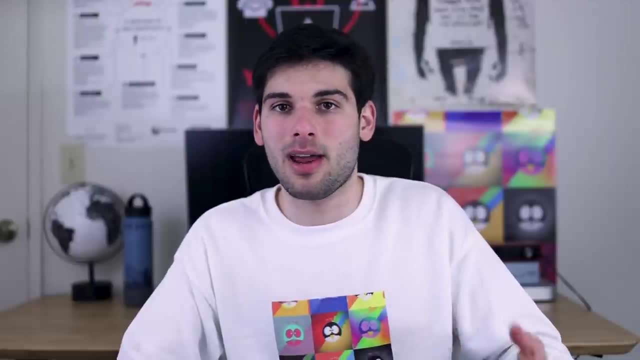 and the latest version of Edge actually isn't terrible. It's improved quite a bit, But Brave and Firefox are better options, as well as the Tor browser. We'll talk more about these browsers and your different options down the road, but for now just avoiding regular Google. 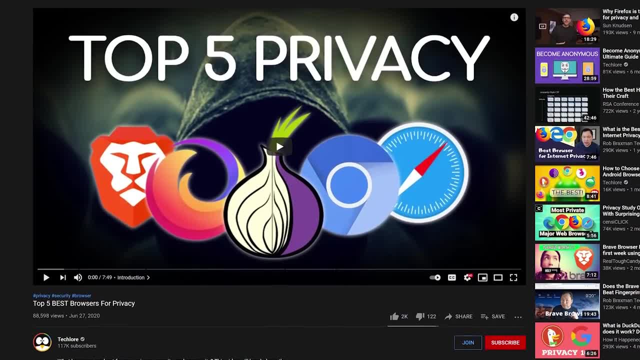 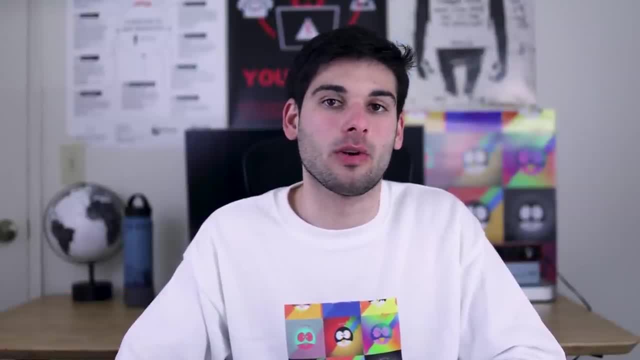 Chrome is a good first step. We have a top five browsers video which goes into your options and the pros and cons of each one. Similar to your browser, your search engine also has the capability of tracking everything you do on the internet, which major companies like Google do. 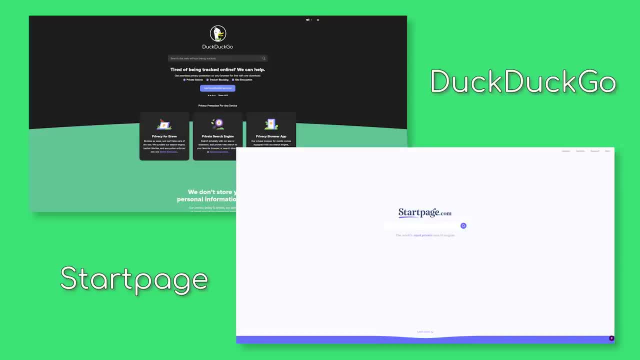 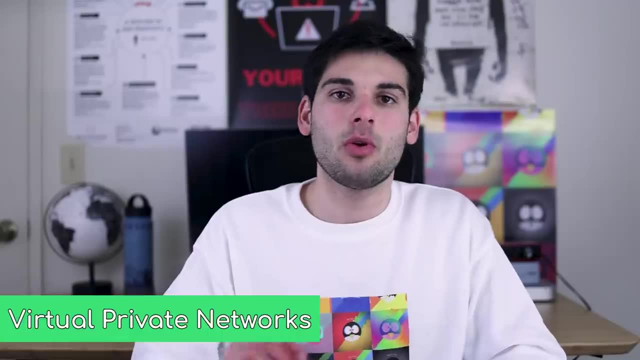 The two mainstream recommendations are DuckDuckGo and Startpage, So see if you can implement one of those within your browsers or use something else with privacy and open source in mind, like searchme. Your IP address uniquely identifies you on the internet and it's 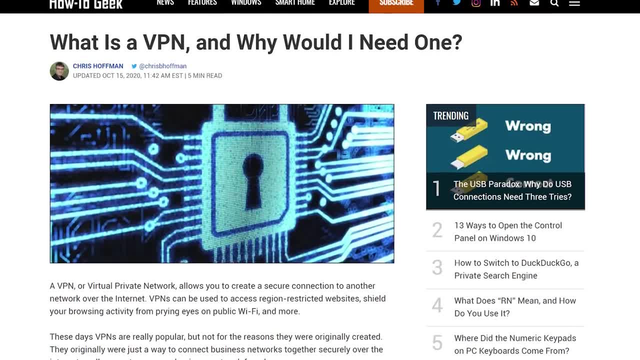 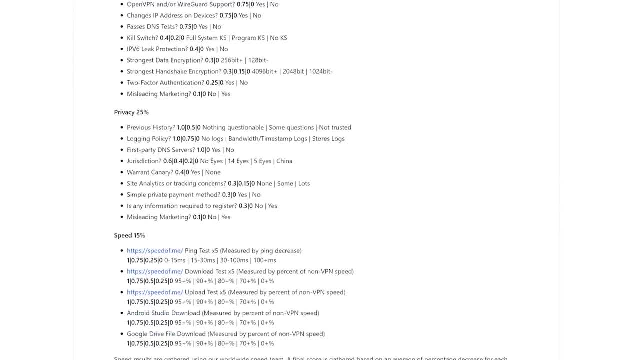 used by websites to track you. A simple way to prevent this is by utilizing a trusted VPN provider to handle your web traffic. As for which VPN to choose the goal in question, We do systematic community-driven VPN reviews on our channel. I'll leave. 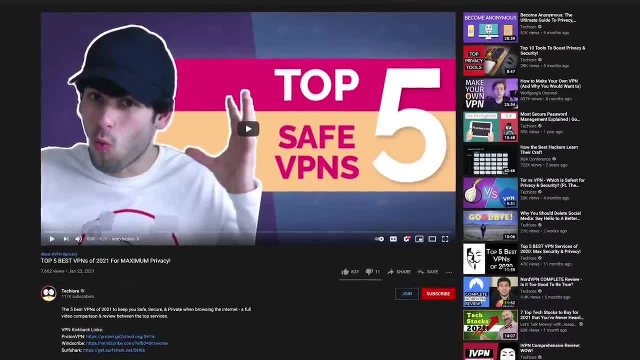 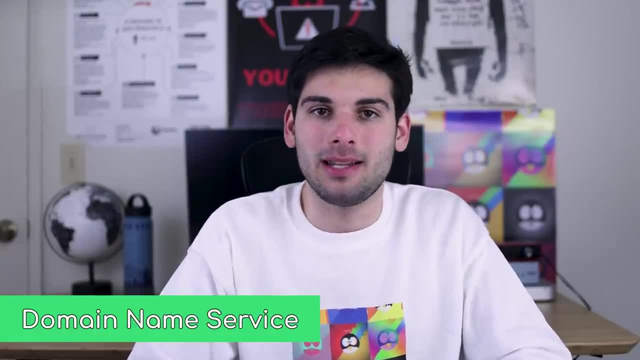 our most current top five best VPNs- video as a card and in the description. We also have all of our open source tools on our website, including a chart where you can directly compare different services. DNS is a domain name service and they are like a phone book for the. 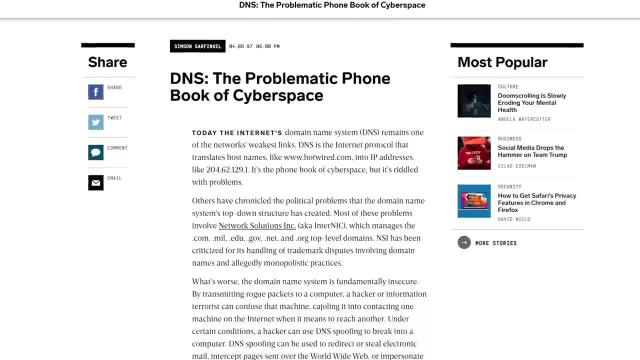 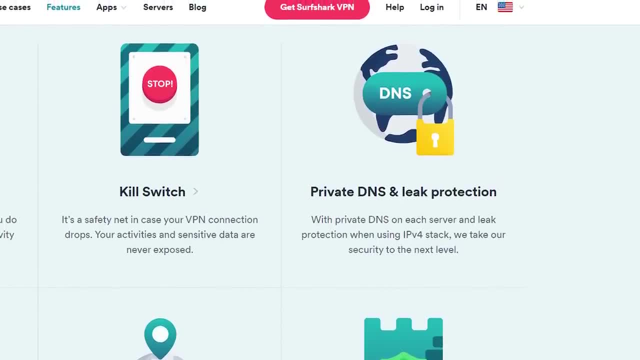 internet, directing you to the sites you visit every day. The problem is: most default DNS providers track your browsing, so use a DNS provider with privacy in mind. If you're using a VPN service, it likely includes its own DNS server, meaning you don't need to worry about this. 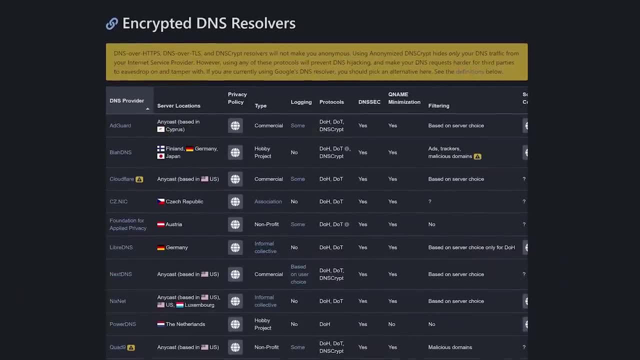 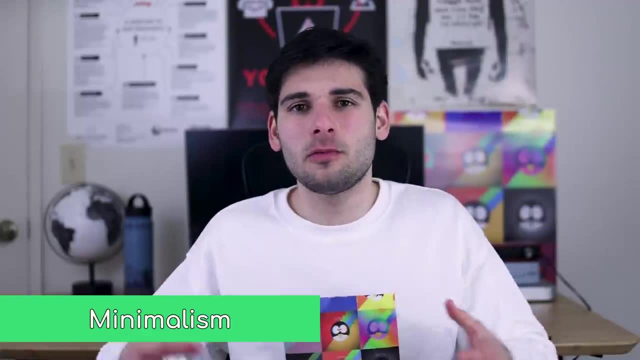 If you aren't using a VPN, check out the DNS servers on Privacy Tools IO and manually set them on your device. You can also utilize some browsers that utilize other DNS improvements if you choose to. This is brought to you by, But less is almost always more when it comes to security and privacy. We actually just covered. 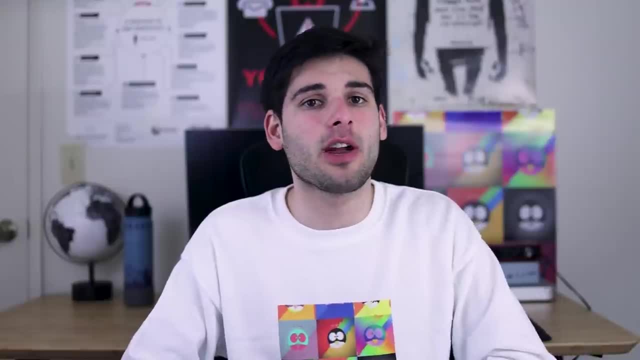 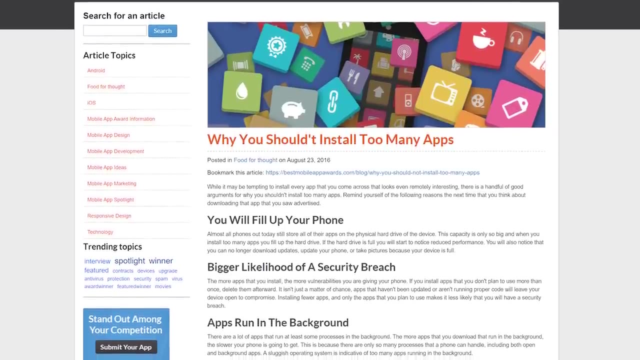 this in a recent video. Go check out our minimalism video. Each additional program and setting you utilize increases attack service and the possibility of abuse with your personal information If you're a person with a never-ending list of programs that you mostly never use. 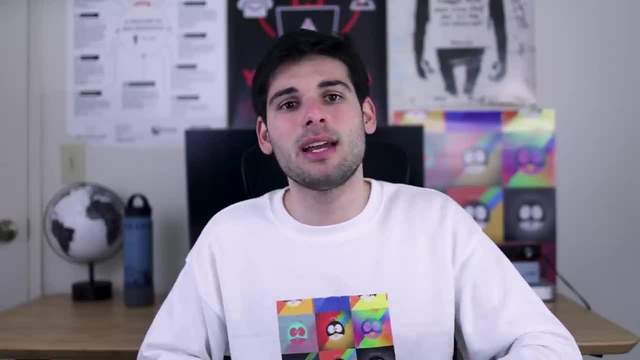 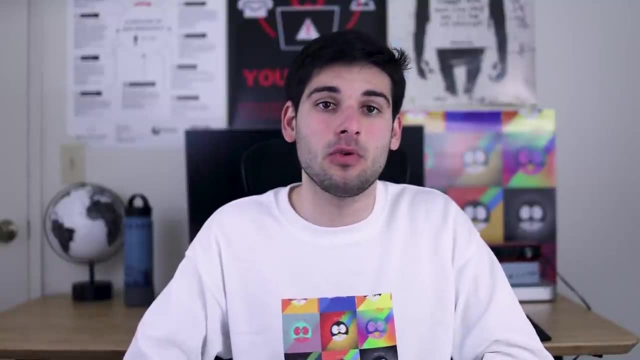 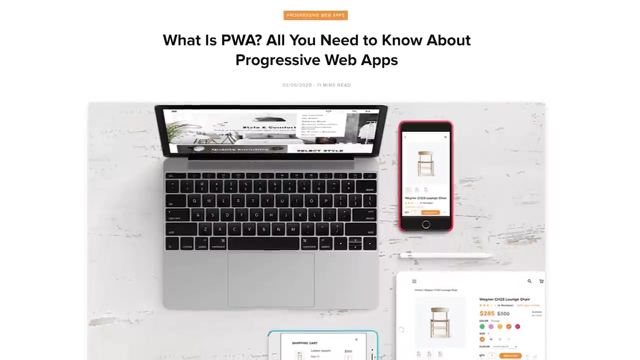 they are likely not just doing harm in the background with your data, but also negatively impacting storage space and power consumption. So delete them or, for the bloatware, uninstall as much as you can. Some programs like Discord have progressive web apps, so if you can utilize the web application within your browser and it'll. 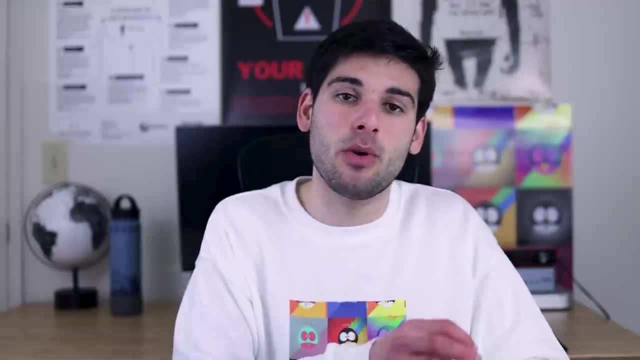 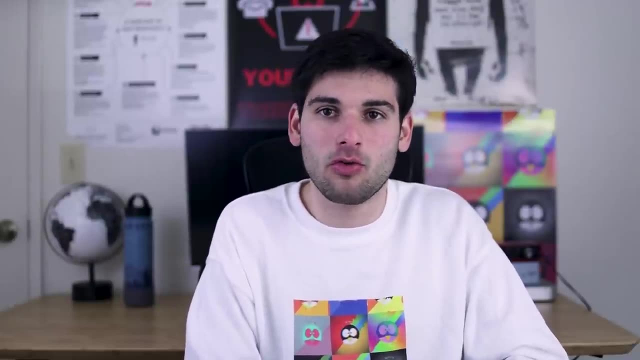 function like the program. it's a great way to separate the program and keep it within your browser, which is typically safer and gives you more finite control of what it can do Outside of programs and settings. try to frequently clear data you don't need. 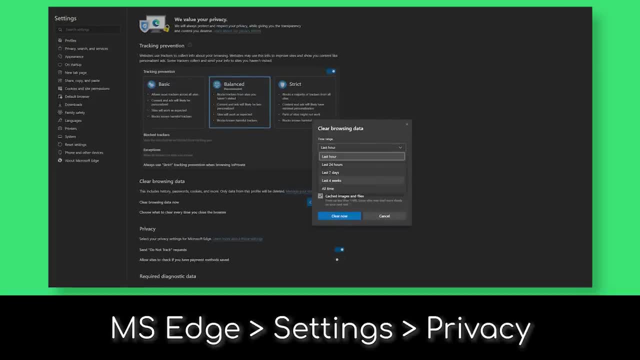 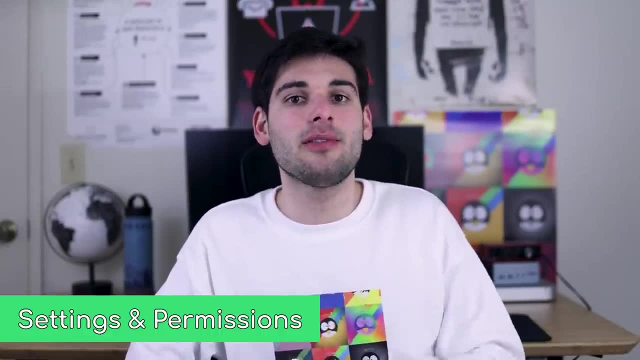 like old system logs, temporary data like browser cache, history and cookies, and any sensitive content that doesn't need to be on your computer 24-7.. Tying into minimalism, there are lots of settings on Windows and its program you may never use and are pointlessly collecting data about you as an individual. 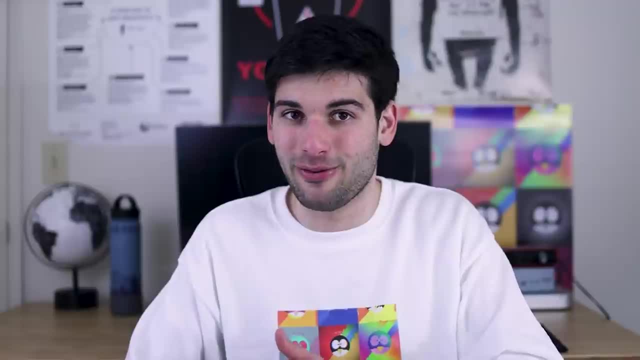 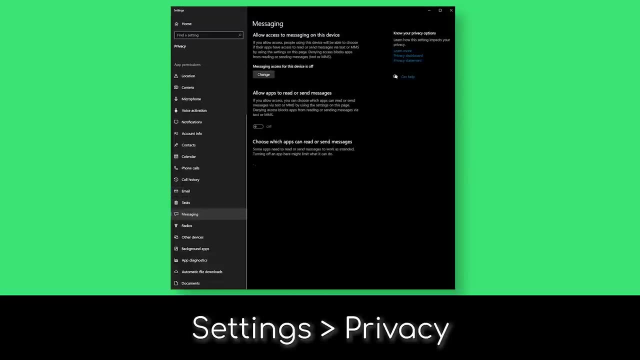 The general rule of thumb is: if you're not using it, turn it off. This may include things like Cortana- which, come on, does anyone use- And there are dozens of settings and features inside the Windows setting app I recommend disabling. Make sure to be thorough and double-check every. 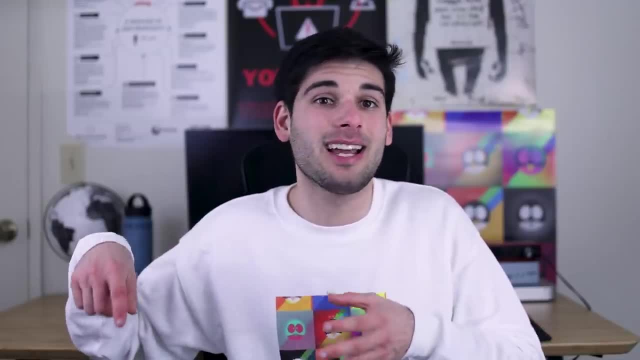 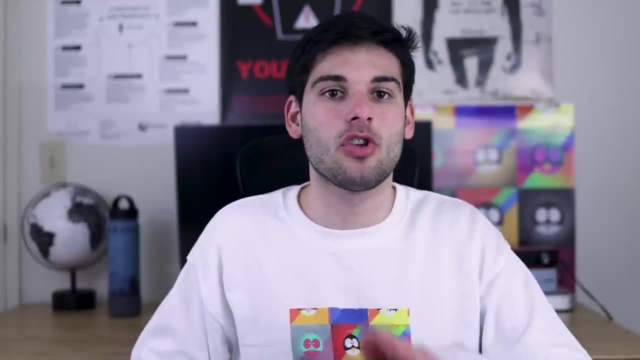 setting. Do not forget to go through each individual program setting as well, to ensure nothing is needlessly tracking you on a program basis. And on a similar note, program and OS permissions should not be used in the same way. If you're using a program that is not, 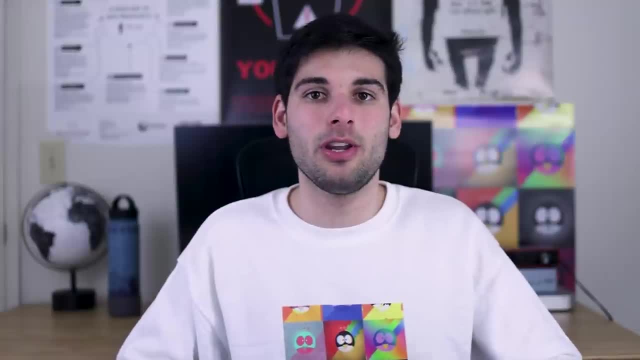 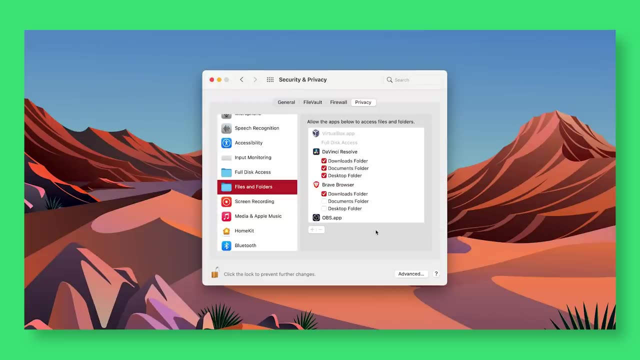 be taken lightly. Unfortunately, in 2021, Windows is still kind of stuck in the past by not requiring individual permissions from programs to do certain things. Gosh man, Mac OS spoils you with this, So do what you can. There are some basic surface-level settings: you 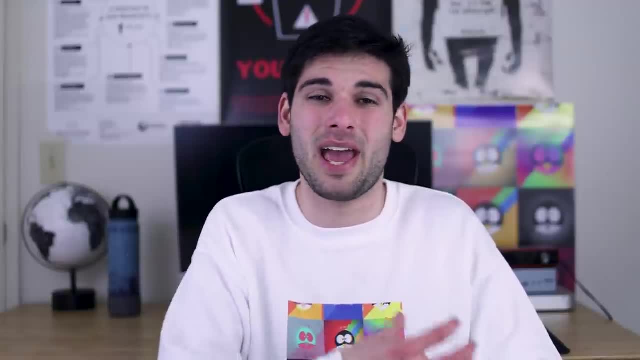 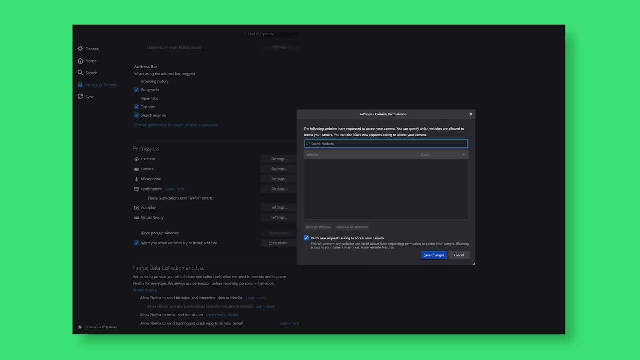 can work with. some programs may have settings that stop the program from performing certain actions, and the best way to control this is using progressive web apps when they're available, because at least your browser does have some form of permission control. Most things you read about online, like the newest Windows. 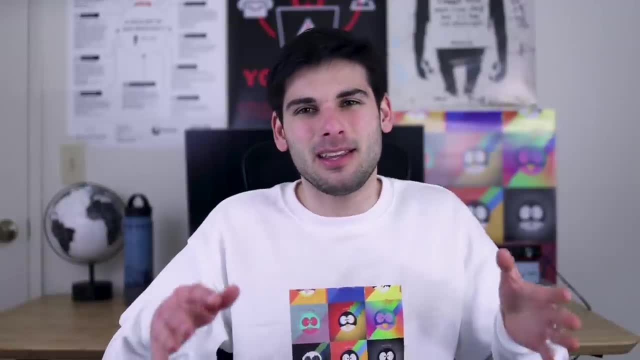 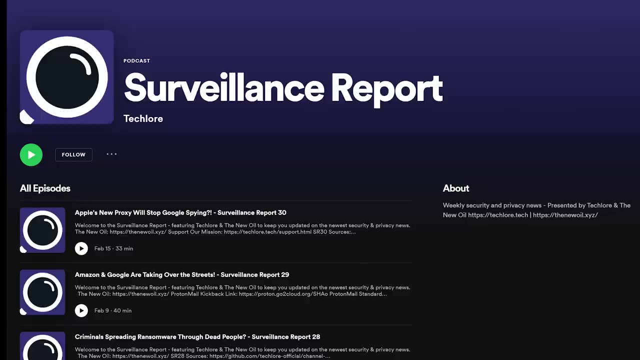 exploits are almost always patched through updates. The best thing to do, as annoying as they are, is to utilize automatic updates for your operating system programs and drivers. To keep up with the newest updates and concerns for all operating systems, check out our weekly news, podcast, Survey and Support. 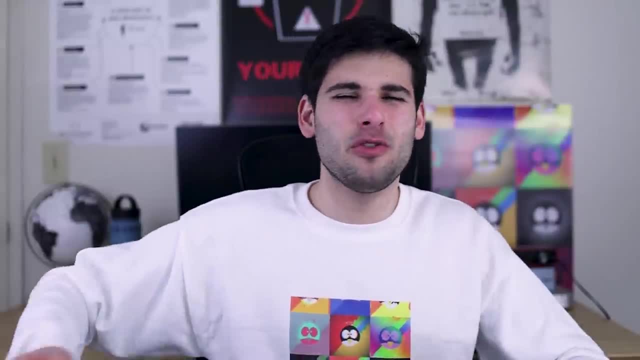 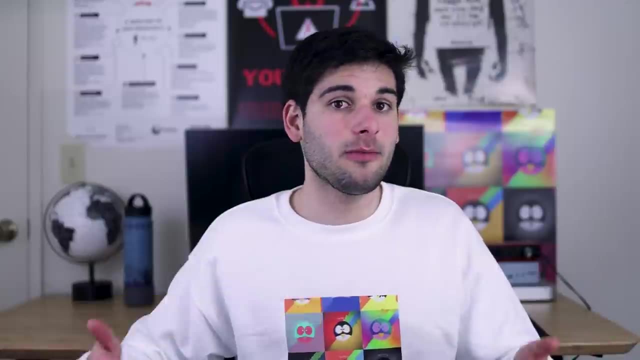 And that's the end of Zone 1.. Let's go ahead and move into Zone 2.. FOSS stands for Free and Open Source. This means the software's code is publicly accessible to the community. If you're looking for a free and open source software, check out our weekly news podcast. Survey and Support. And that's the end of Zone 1.. Let's go ahead and move into Zone 2.. FOSS stands for Free and Open Source. This means the software's code is publicly accessible to the community. If you're looking for a free and open source software, check out our weekly news podcast. 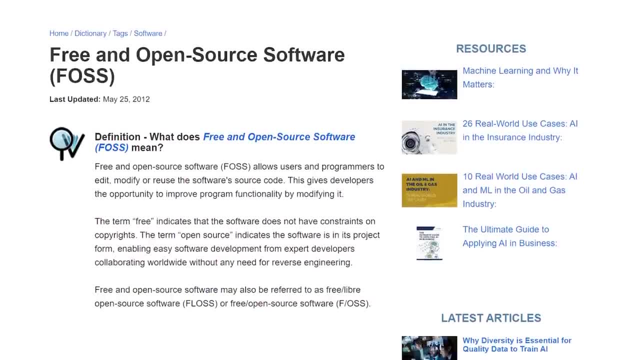 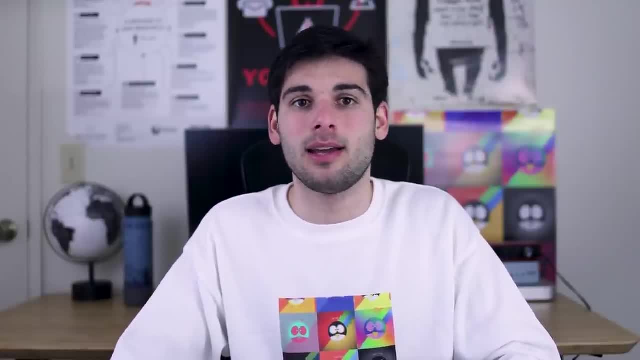 Survey and Support. This means the software's code is publicly accessible to the community. This also ensures you can verify the security and privacy behind the software. We have a video covering this more thoroughly. In general, I'd advise moving from proprietary to FOSS programs as much as you can. 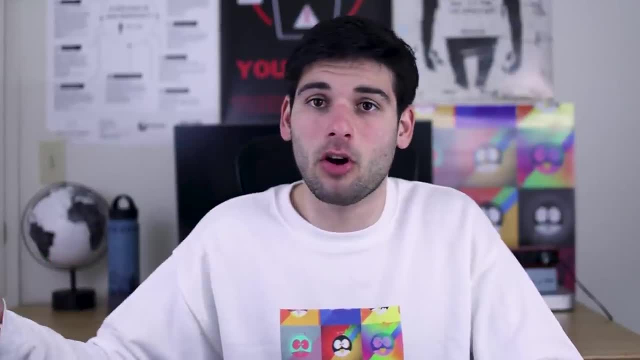 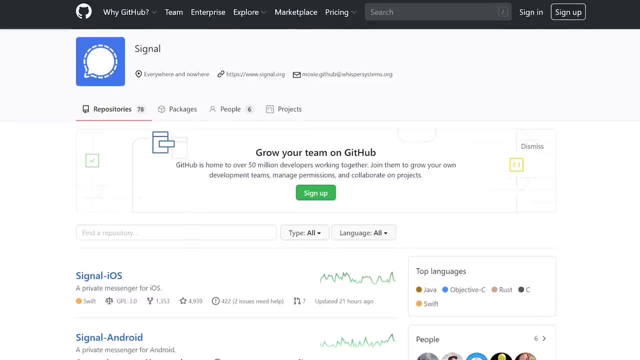 Yes, Windows itself is proprietary, but improvements are improvements. Some VPNs, like ProtonVPN, iVPN and MOLVAT, have open source clients. Signal has a desktop program that's open source and even things like Screenshot. tools. 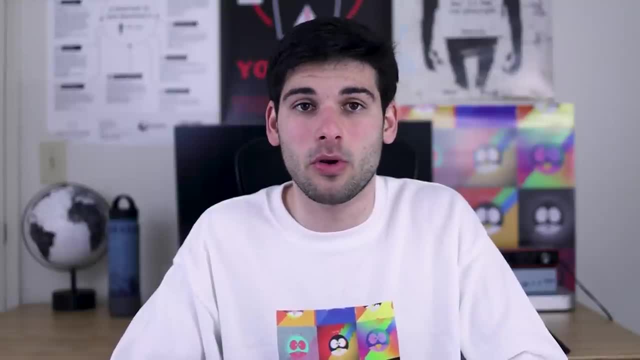 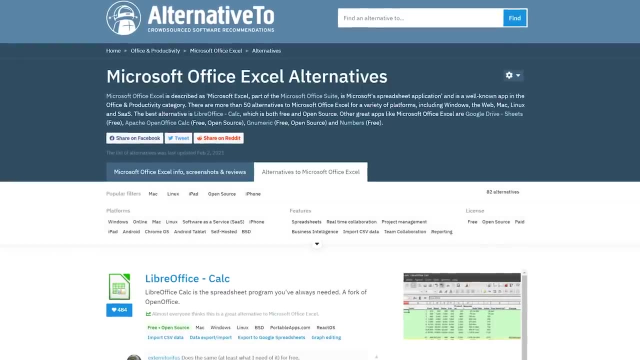 such as GreenShot, are open source tools that you can utilize on your computer. Just go through your list of programs- One of them is Screenshot- One by one, and type each of them into Alternative2.net with the open source filter and see if there's something you can switch to. 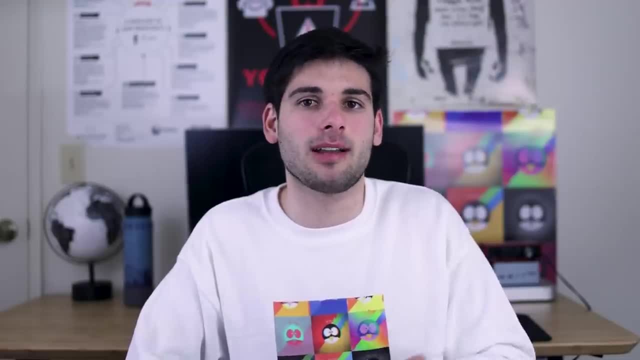 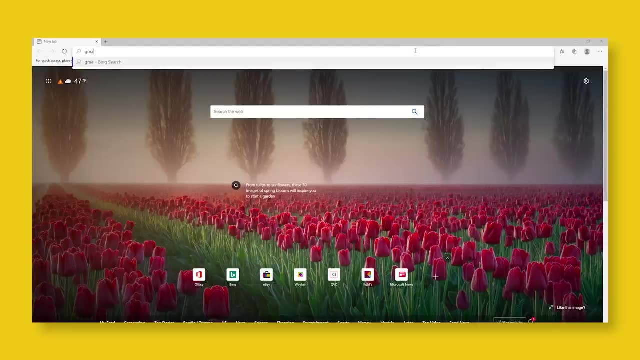 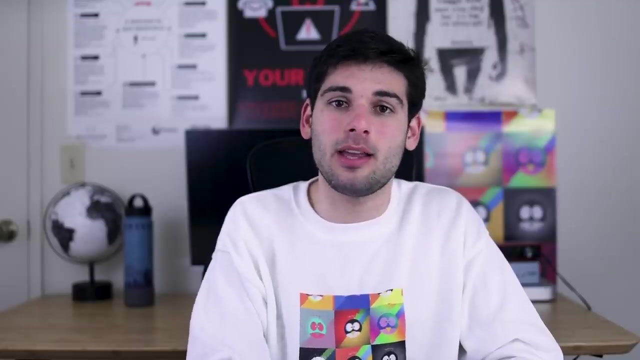 FOSS will typically honor you and your data better than proprietary solutions. Your computer is ironically, used less for communication than you might think, at least in the context of direct contact with another individual or individuals. It's recommended to keep email in your browser to add an additional safety layer between an email. 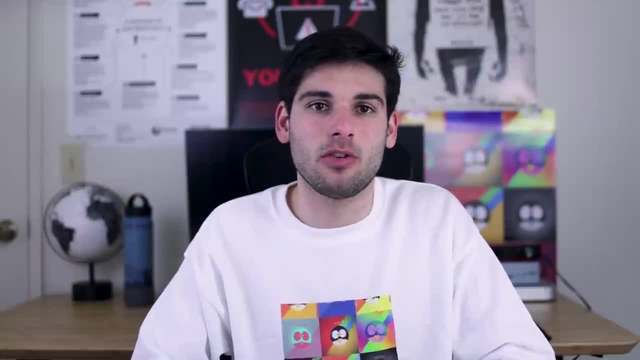 and your operating system In regards to what email provider to use. well, we have a nice video on that. With direct messaging first, I recommend switching to something built from the ground up to protect you, like Signal or another messenger listed on our site's resource page. 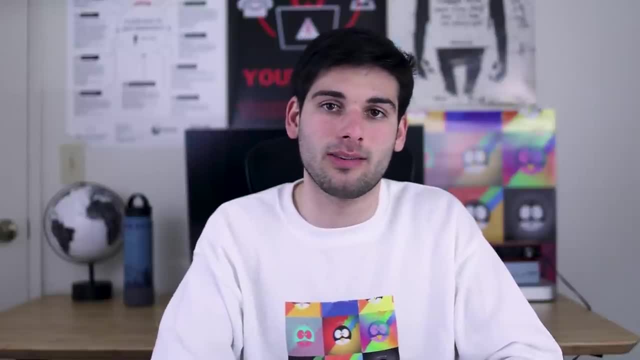 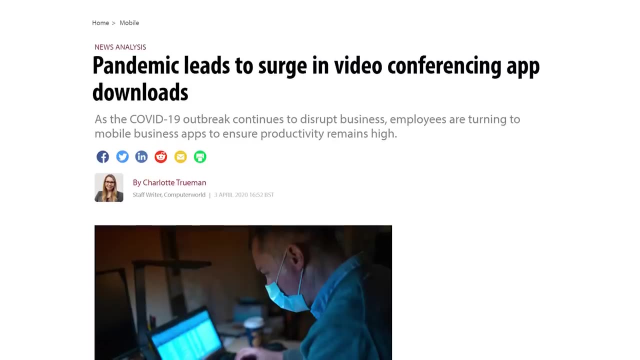 But if you are stuck using something like Facebook Messenger or WhatsApp, enable end-to-end encryption where you can and try to keep the program off of your computer, keeping them inside your browser instead. Thanks to the pandemic, video conferencing is the next big thing, and like direct messaging. 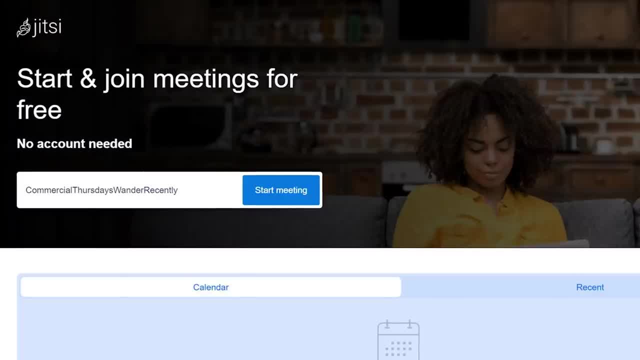 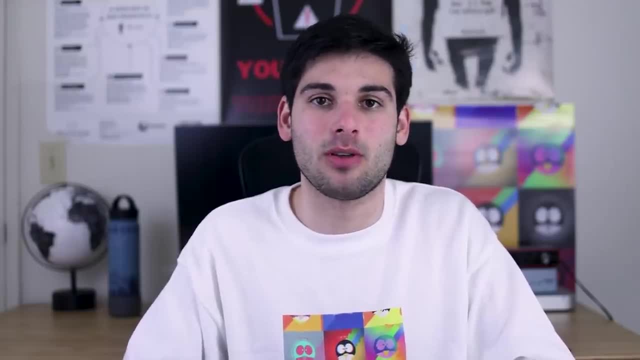 the first goal is to move to things that naturally respect you. Jitsi- CalixMeet- an instance of Jitsi- and BigBlueButton are all good alternatives to Zoom, Skype and other options, And again, like direct messaging if you are stuck on a not-so-great platform. 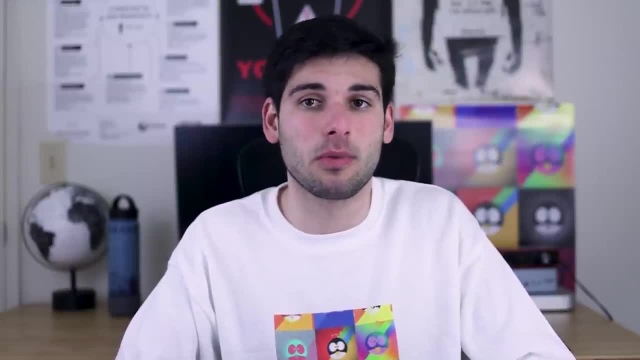 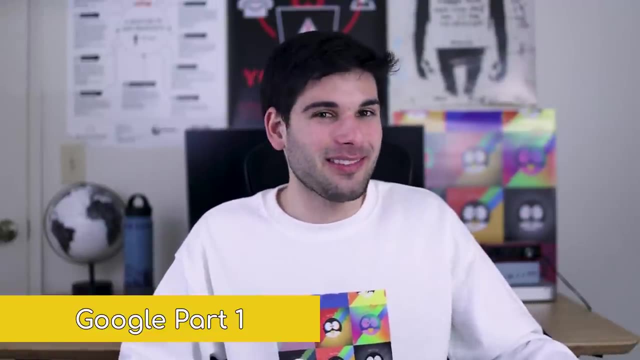 the goal is to keep it inside your browser when possible and avoid using the program. We'll talk about virtual machines later in the video, and that will be another tool that you can use. in regards to these, Avoiding Google is a great step for controlling your data. 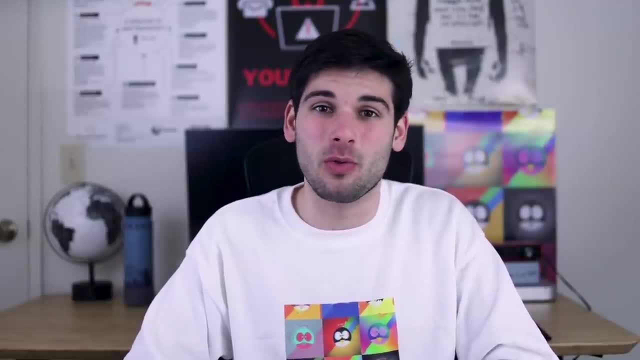 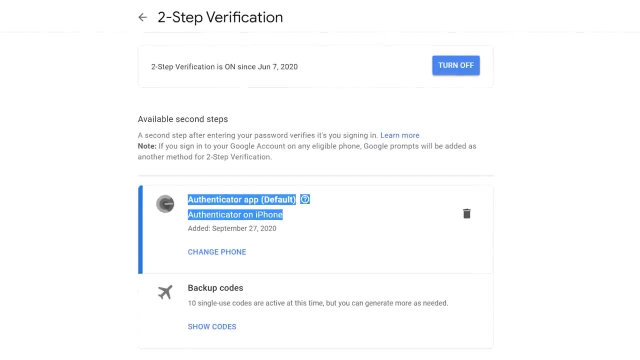 as Google is not a privacy-friendly company in 2021.. Newsflash For Zone 2, disable as much as possible related to Google in your My Activity page and ensure you're using 2FA and have properly secured your account. We have a guide going through this. 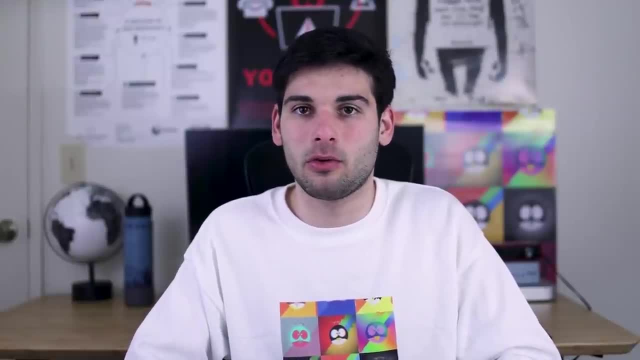 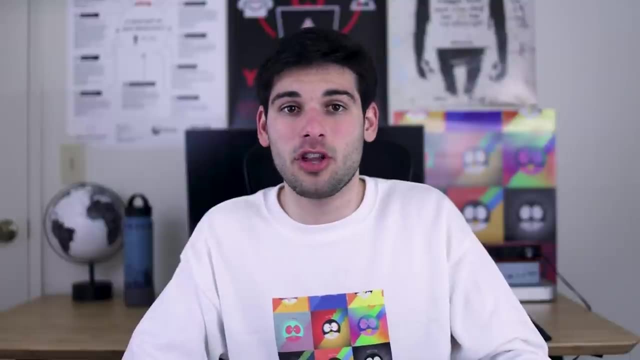 Additionally, being less reliant on Google is equally important. so switching to Brave from Chrome gives you a less-Googled life and you don't need to go raw turkey to make improvements. Switching your default search engine, turning off everything in the My Activity page. 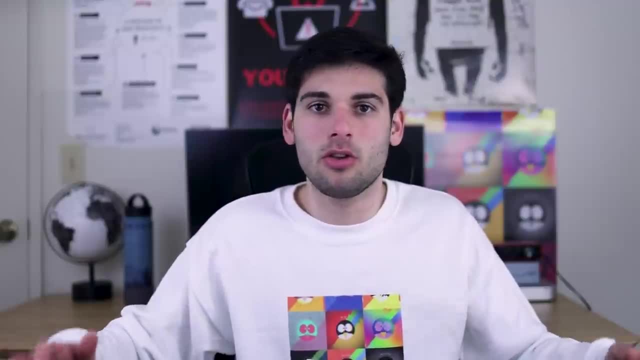 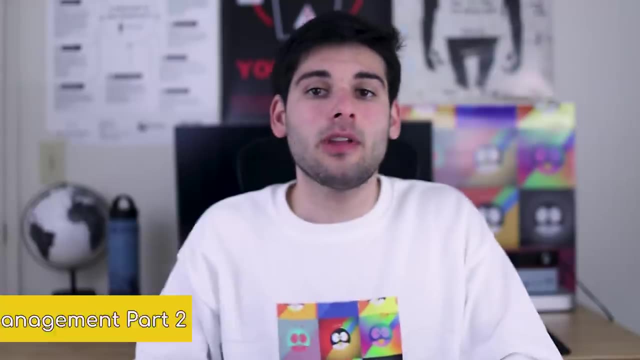 and switching to Brave from Chrome is absolutely huge and should take you less than 15 minutes to do, with almost no effect on your day-to-day life. So just do at least the little things if you can Outside using strong and unique passwords, which we covered in Zone 1,. 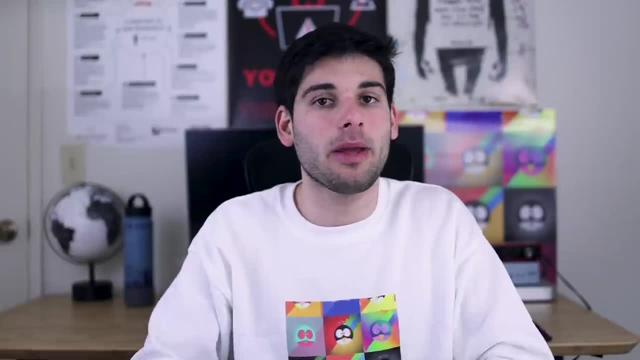 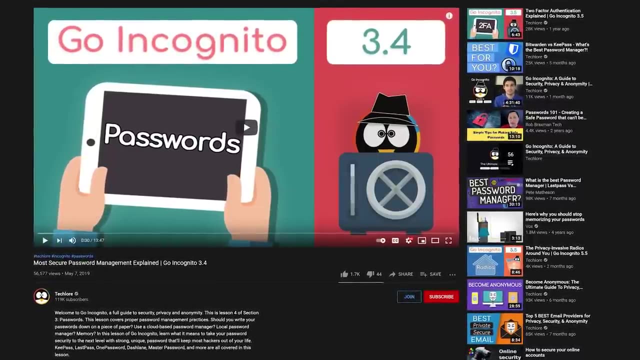 where and how they're stored can be incredibly important as well. Password managers are a commonly recommended way to go. We have covered what these are and how to use them in the lesson of Go Incognito, so check out that for a long answer. 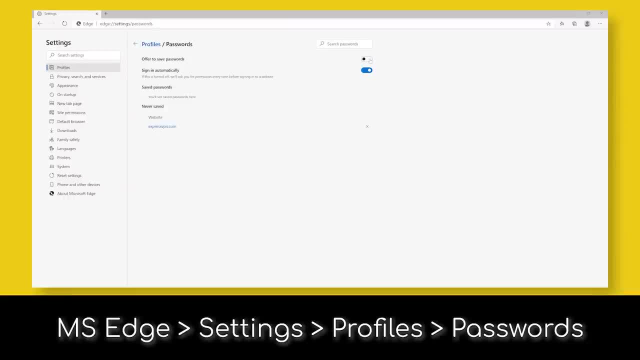 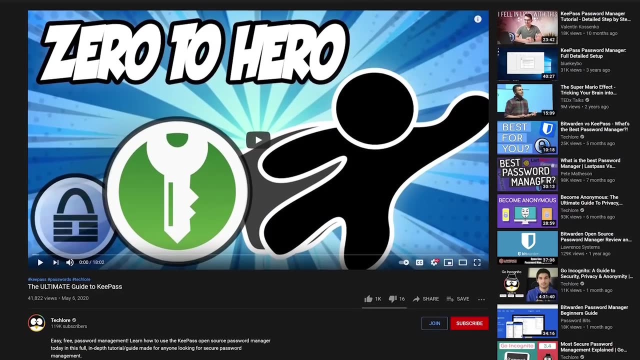 In short, avoid storing your passwords within your browser. If you want simple cloud-syncing between your devices, check out Bitwarden. If you want a more DIY password manager, there's KeePass. We have a whole guide on KeePass on our channel for those who want to learn about it. 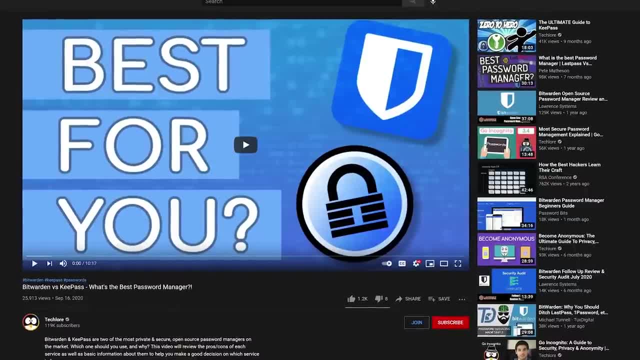 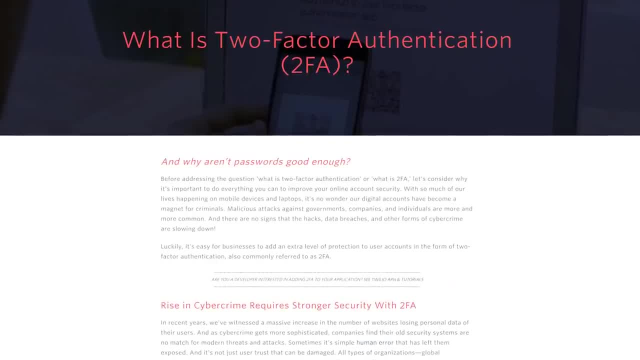 and we also have a comparison video between these two things, So check it out if you want to learn more about these two fantastic open-source password managers. Beyond your password, implementing two-factor authentication is arguably just as important. 2FA combines something you know- a password- with something you have. 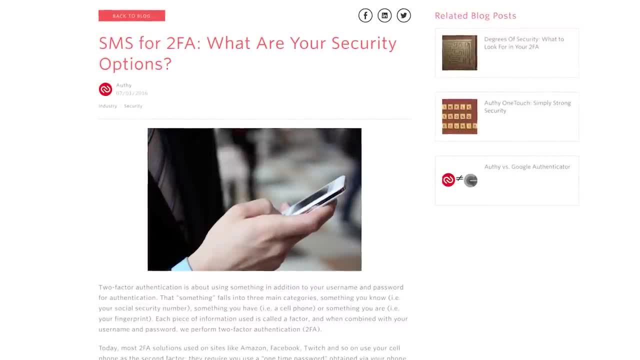 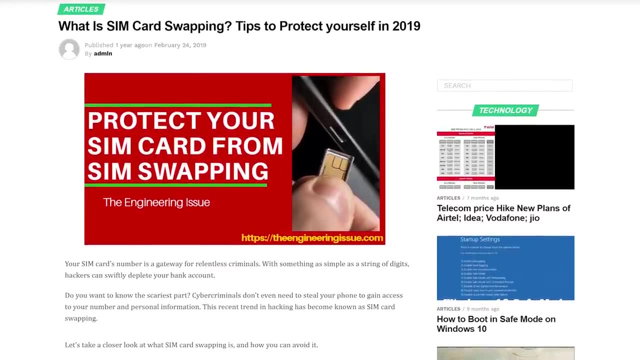 ideally a code generated locally on your device At the very least. SMS 2FA, which are those texts you receive with a code, is better than nothing. But there are a couple issues with SMS 2FA, like the risk of SIM swapping. 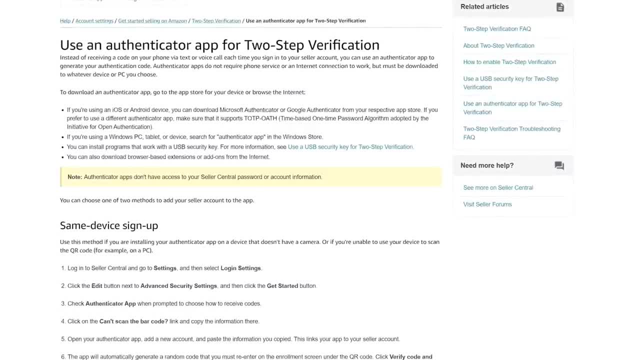 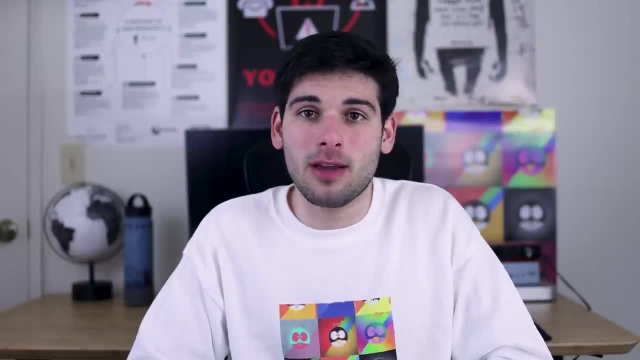 The better and more recommended option is a local authenticator app on your phone that uses a QR code. It supports this, but many do, so look for it and use it instead of SMS when available. If you want FOSS recommendations, Android has AndoTP and Aegis, and for iOS there's Authenticator and Tofu. 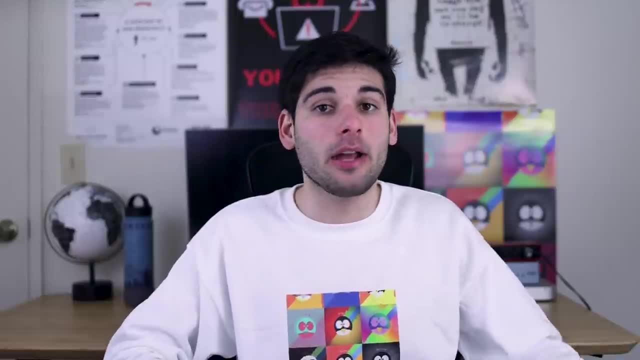 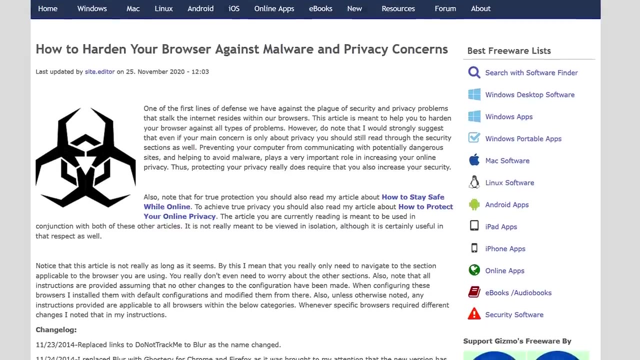 Part 2 of browsers is to take things to the next level. I'd recommend sticking to strictly open-source browsers like Tor, Firefox, Brave and Chromium and properly hardening and configuring each browser for the absolute safety. We cover Firefox hardening in Go Incognito. 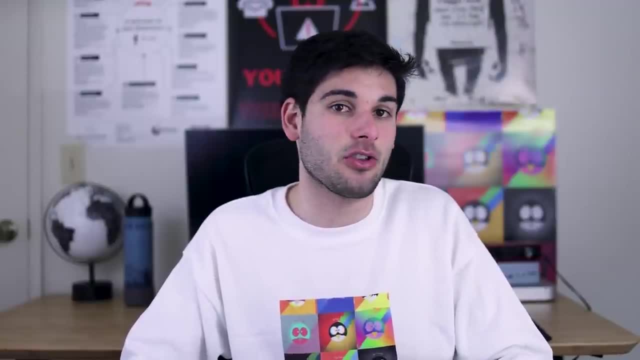 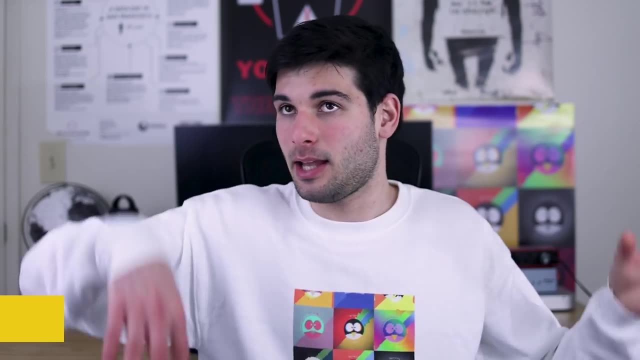 and Brave, mostly requires just basic settings, toggles, as it does much of the work for you out of the box. And yes, you do have to get rid of all the crypto crap. Tor should not be messed with outside the basic safety sliders. Then we have radios, which apply to anything that gives off a signal on your computer. 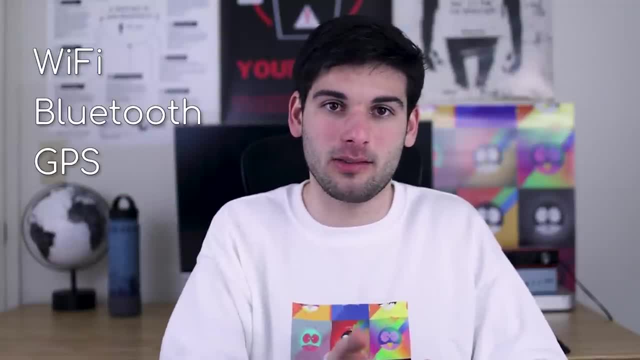 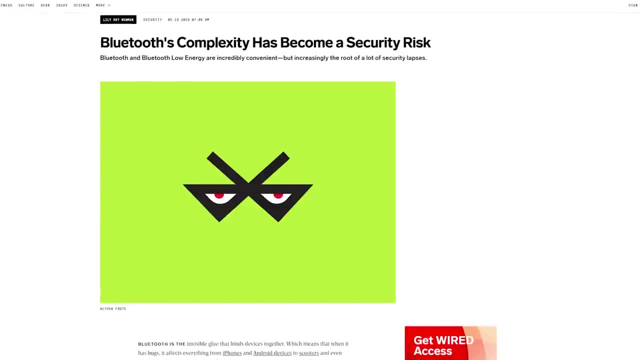 This means predominantly WiFi, Bluetooth and GPS. We'll cover the more extreme solutions in Zone 3, but for Zone 2, try disabling Bluetooth and location services when they're not being used. Bluetooth for one can be an insecure protocol, not to mention Bluetooth being an instrumental tool. 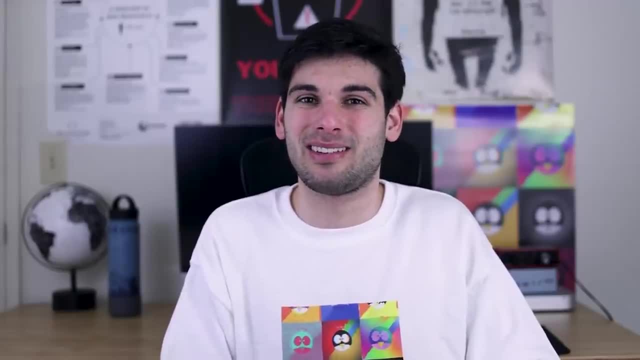 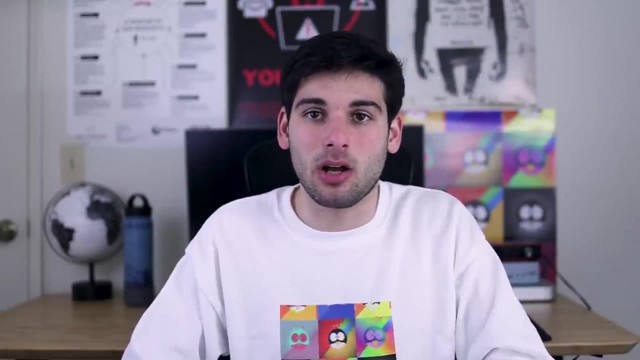 to track your movements. This is a smaller concern on a computer, as it's not traveling around town like your phone, most likely, but it's still a good practice. The general rule of thumb for radios is if it doesn't need to be on. 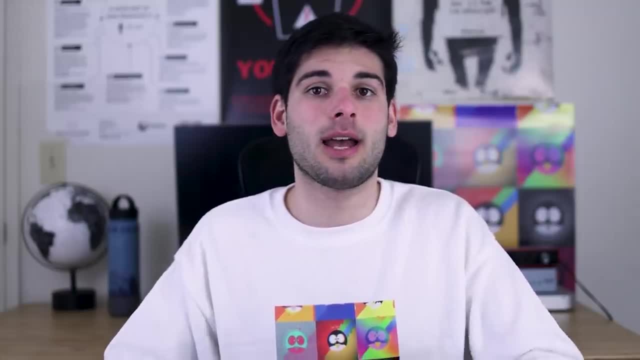 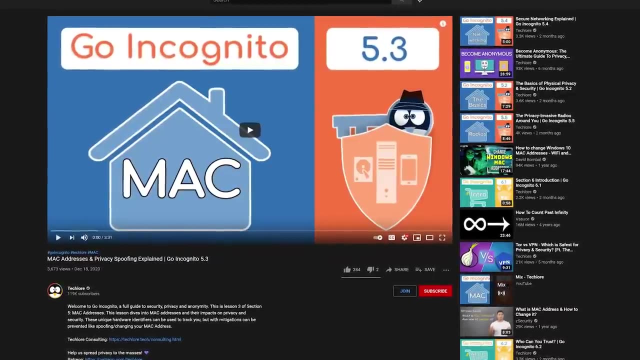 the last radio you should be aware of is WiFi. Your device broadcasts a unique ID, called a MAC address, which can be used to track you. We covered how this is done and how elaborate this can be in Go Incognito. In short, consider randomizing your MAC address. 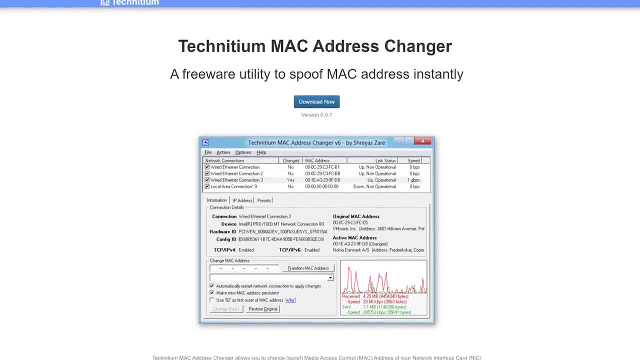 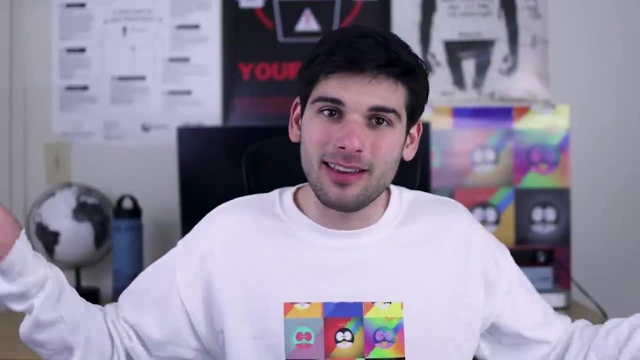 which I believe is now an option in Windows, or you can use a tool like TechNative. Now Windows offers something very neat: Multiple user accounts. Well, most desktops do nowadays, But yeah, Windows has this. You can use these to compartmentalize or separate different aspects of your life. 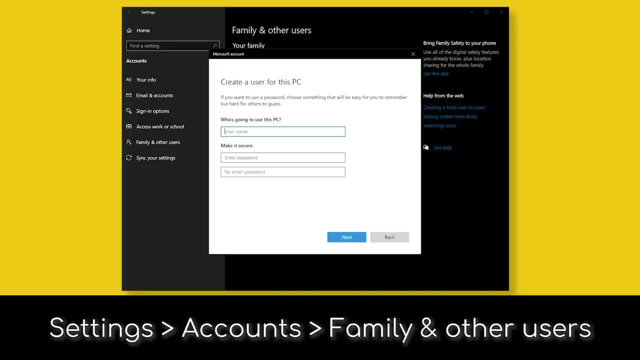 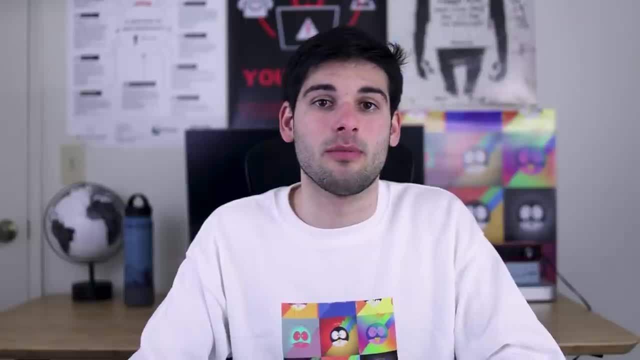 Maybe you have a business account, a school account, a dating account and then your personal account. The goal here is to separate aspects of your life that don't need to be intermixed Additionally for those who want to go above and beyond. 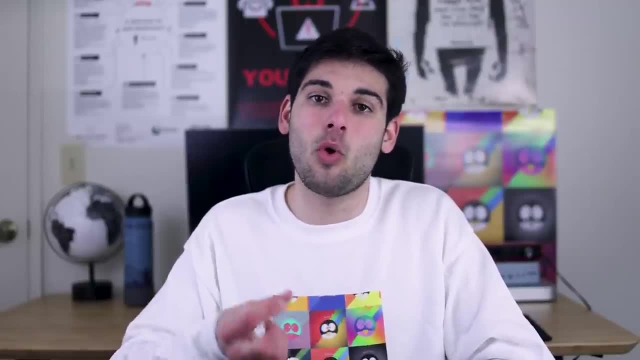 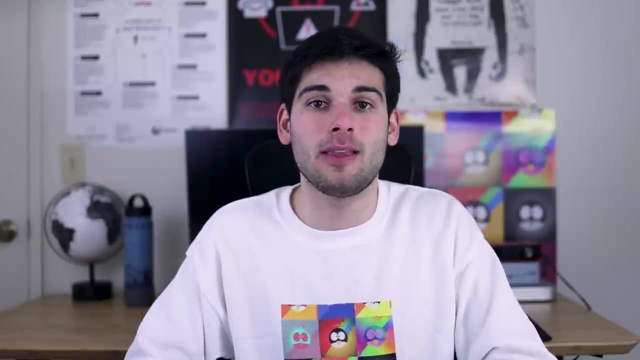 you can have an administrator account and a standard user account and stick to only using that standard account for your daily usage. as a security perk, This prevents any of those things from happening- Rogue applications, malware or anything else from utilizing that administrative access. 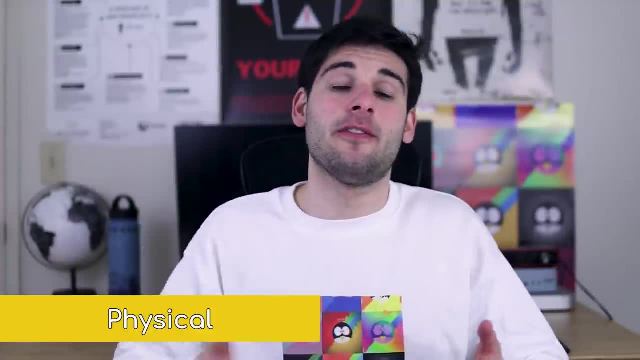 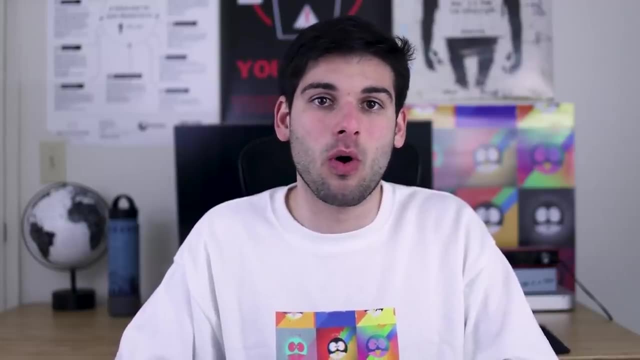 to damage your system. And then we have some extra steps in regards to physical protection of your computer. Make sure your BIOS has a password. Consider locking your desktop or laptop to a desk or wall, if this is an option. I'll leave some products below. 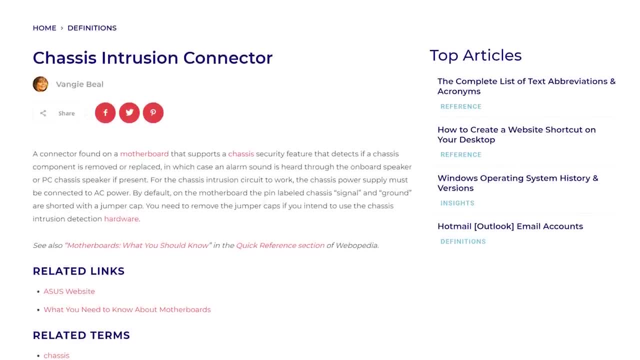 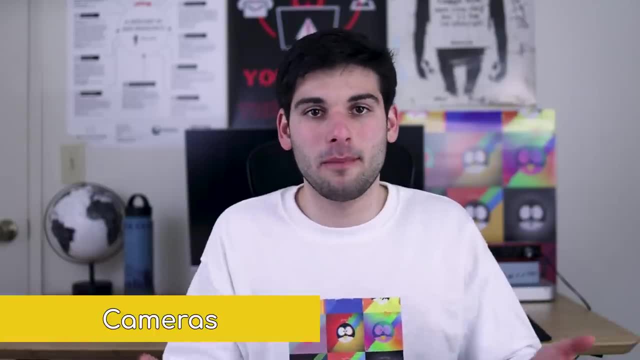 And some motherboards have intrusion systems which detect if the computer is opened up. If you want to go above and beyond, there are projects like Coreboot, which may be able to replace your BIOS's firmware. Most people are aware of this one, but covering your cameras can prevent the theoretical problem. 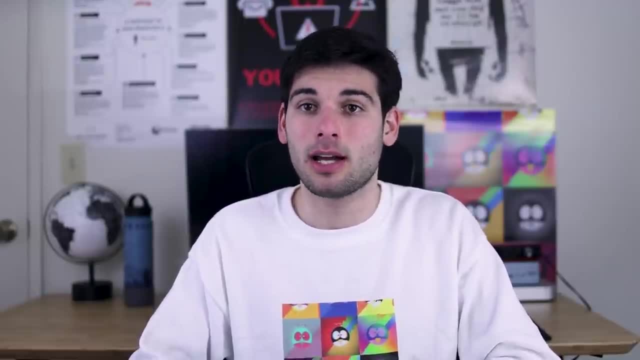 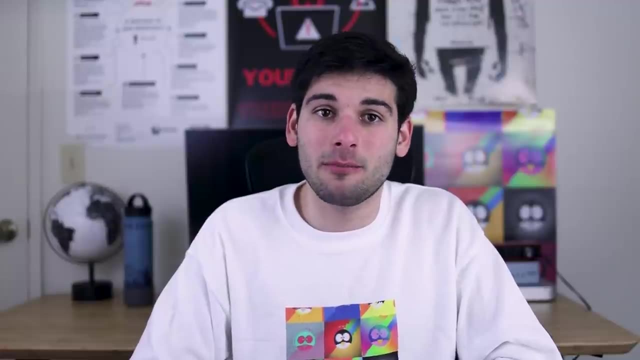 The theoretical camera hack where someone spies on you through your camera. Cover them up If you never use your cameras and don't want to just use tape. A nice thing with desktops is they normally don't have a webcam like laptops do. 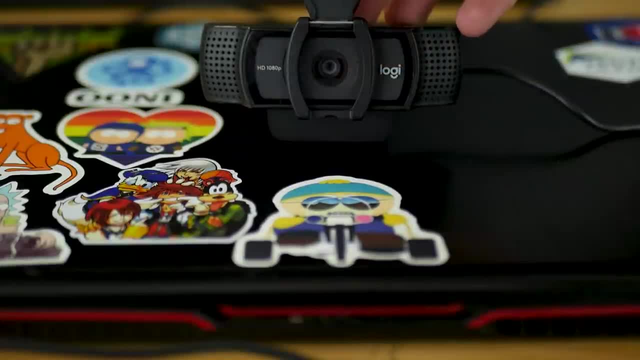 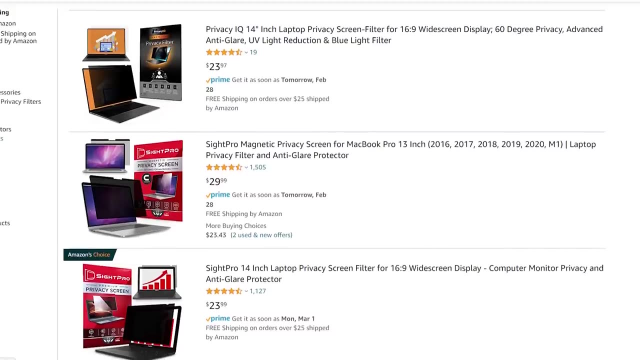 so you can instead rely on an external webcam with a great amount of peace of mind once it's unplugged. And the last step for zone 2 is utilizing a privacy screen protector. These make it so it's very difficult to view your device's screen from side angles. 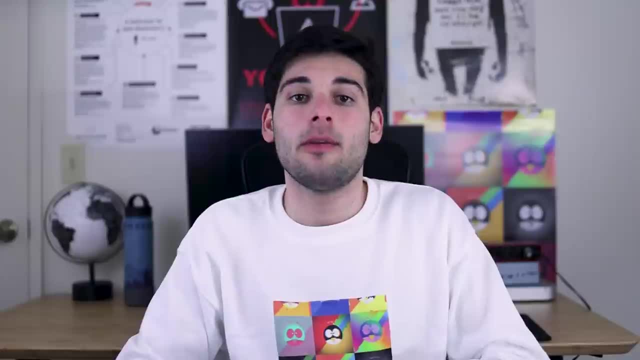 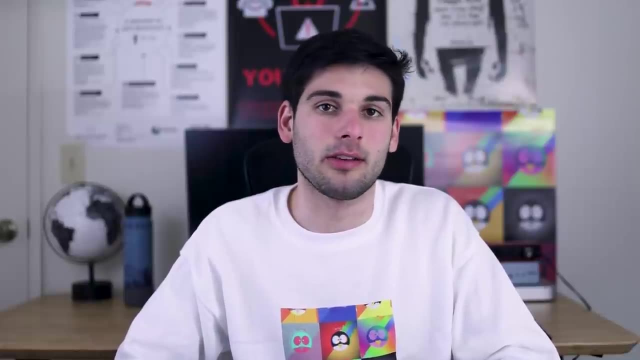 protecting your personal information from snoops and shoulder attacks. The main downsides to these is they can affect the display quality a little bit, just an FYI, but most people probably won't notice unless they're working in a color sensitive environment. This is it everybody. 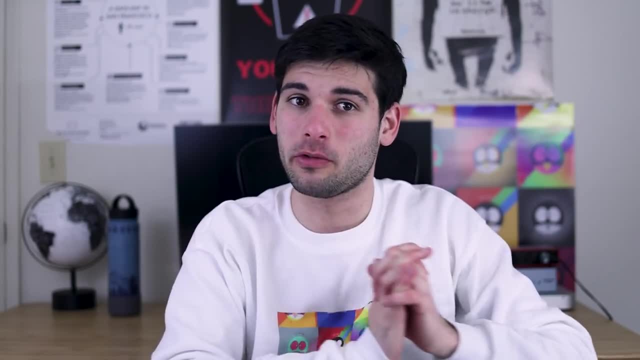 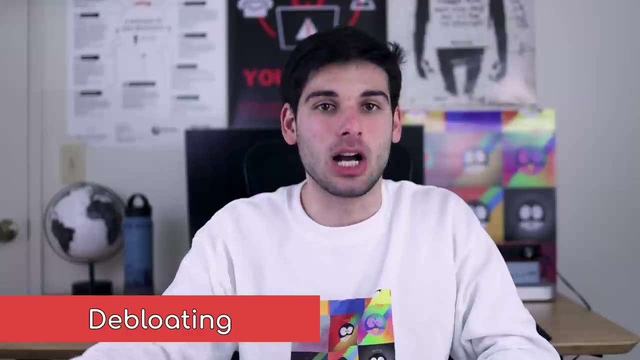 Zone 3, and, like I said earlier, this is for the extreme users looking for the utmost security and privacy on their devices. The next level of minimalism is removing the gunk that's built into the operating system itself, Even if you turn off all the settings and you've done everything else in this guide. 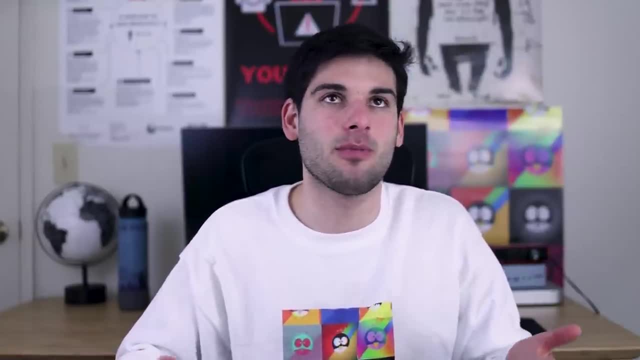 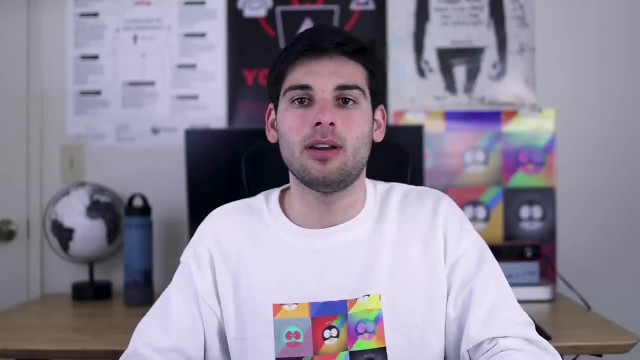 Microsoft will still collect some data about your system. Some is probably an understatement. To mitigate this as much as possible, you can use your phone, Check out tools like Win 10, Privacy and Shut Up 10.. While none of these tools are foolproof and guaranteed to stop all of this data collection. 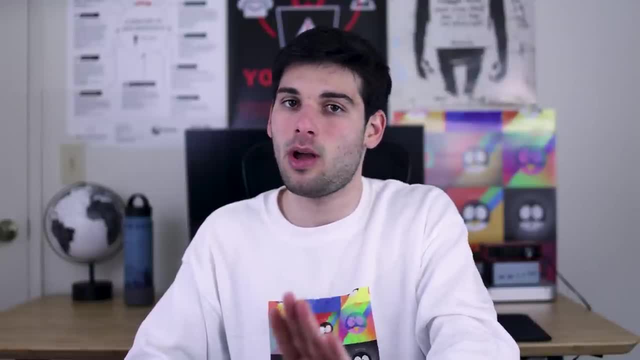 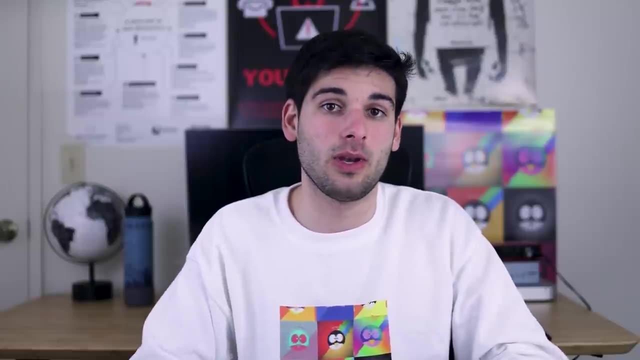 they do attempt to do so. Please proceed with caution. as well as some of the settings in these tools remove things that are very hard, if not impossible, to recover without reinstalling Windows. It's recommended to do a full system backup before experimenting with any of these tools. 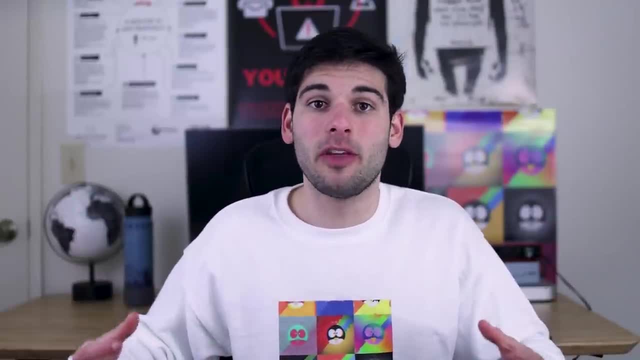 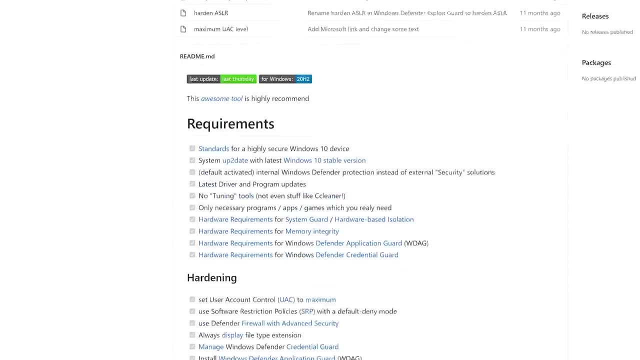 Up next is hardening, and this is pretty much where we're going to improve the security and privacy of Windows through several configurations. This GitHub repo Windows 10 Hardening from beerisgood is a great starting point, taking you through all the different settings and features you can implement to boost. 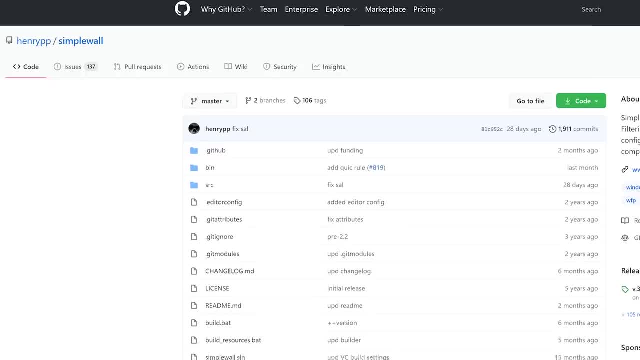 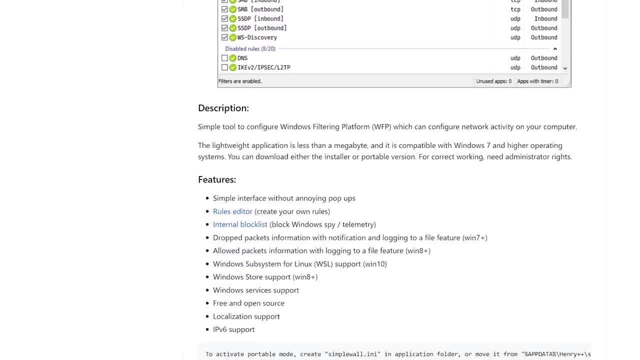 the security and privacy of your system. Additionally, Simplewall from henrypp, which is definitely clearly advertised for advanced users, lets you fine-tune network activity on your computer, which you can use to block unwanted things your system is doing in the background. 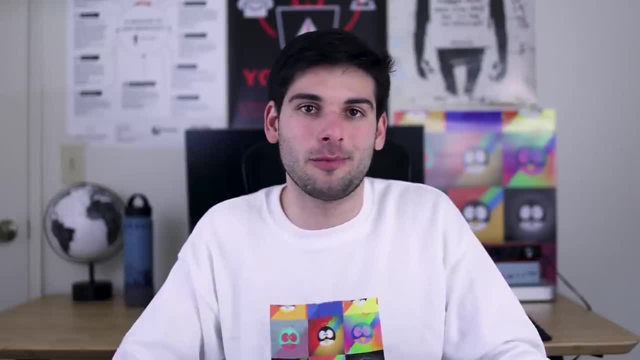 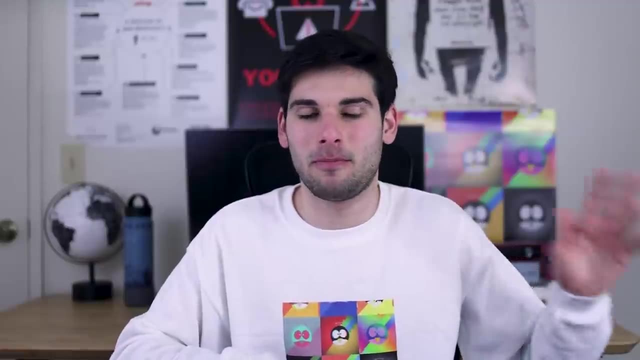 To take Google a step further, you should fully delete it or remove every trace of it on your system, Unless you have some elaborate solution to properly compartmentalize Google on a separate device. But that's an edge case. To repeat Zone 2, if this is all too extreme, at the very least ensure you've handed over. 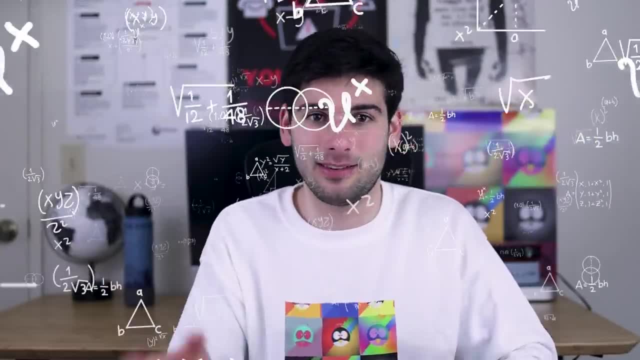 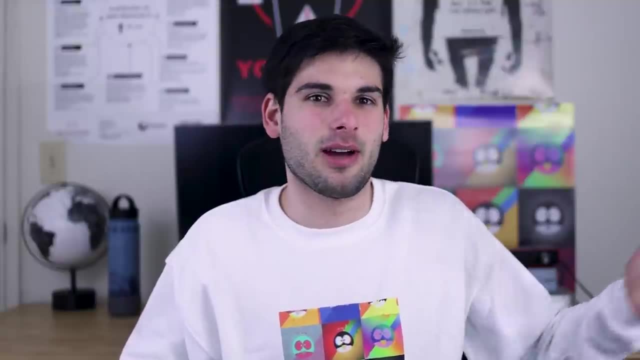 as little personal information as possible to Google. disable the analytics performed by them in the settings. disable as many features as possible. you guys get the point. Go back to Zone 2 if you want to see that again. And, kind of a side note, make sure to delete social media too. 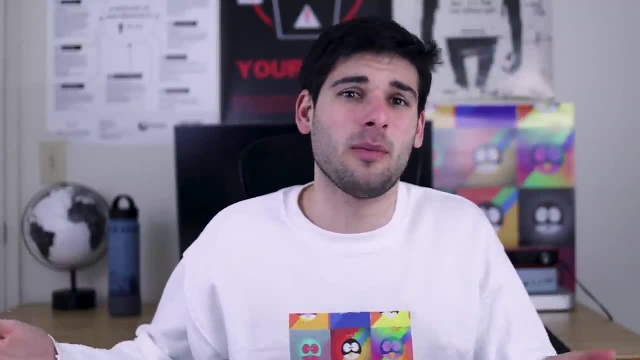 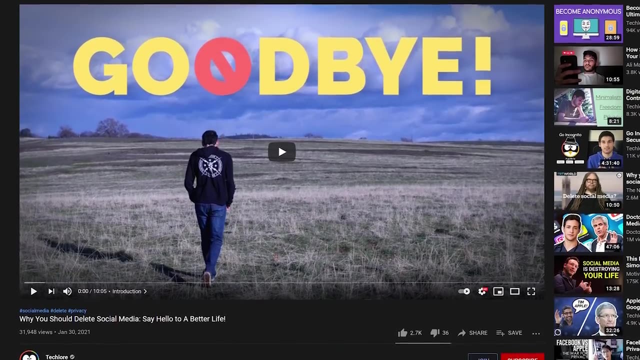 I hope that was a given, but I should specify that Social media should probably be deleted at this point. We just made a video talking about this and how awesome it can actually be. It's not just for privacy. You should totally delete it. 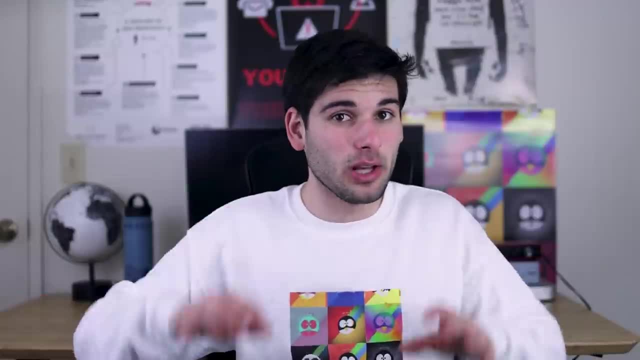 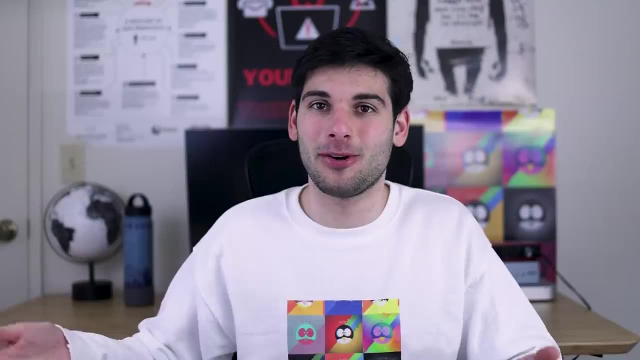 Alright, snip-snip, These are those pesky cameras and mics. If you really don't want them and you want full peace of mind, consider removing them from your computer. Depending on your laptop model, this can be extremely simple or it can be extremely hard. 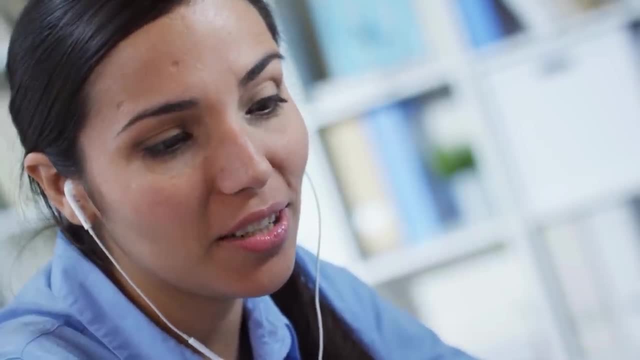 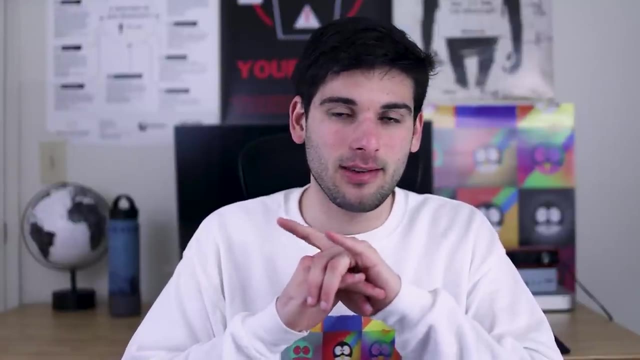 You can also snip the microphone and stick to only using the microphone on your earbuds or an external mic. This is for very extreme threat models, but the option is available. Do note that opening up your device may void its warranty. And finally, obviously this whole video has been about Windows, and as nice as Windows. 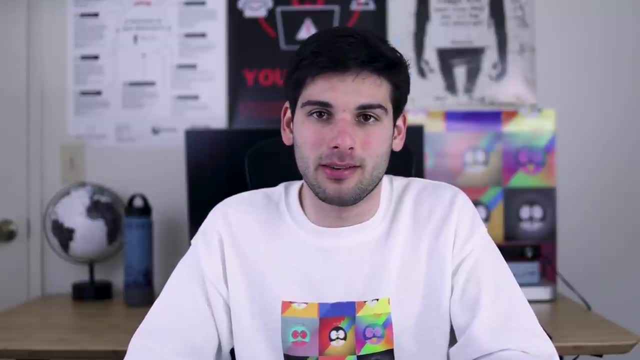 can be. sometimes it can be a little bit of a pain in the ass. So if you have any questions, feel free to leave them in the comments below And I'll see you in the next video. Sometimes it's actually easier to just switch your operating system. 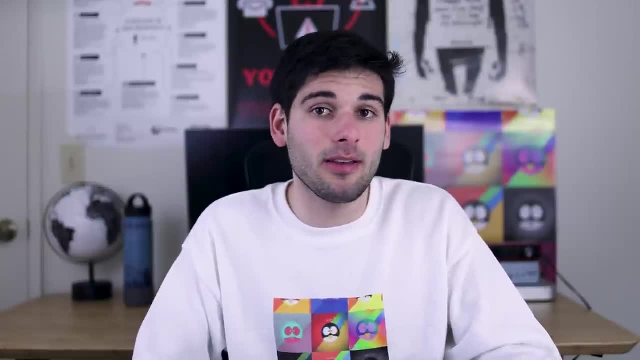 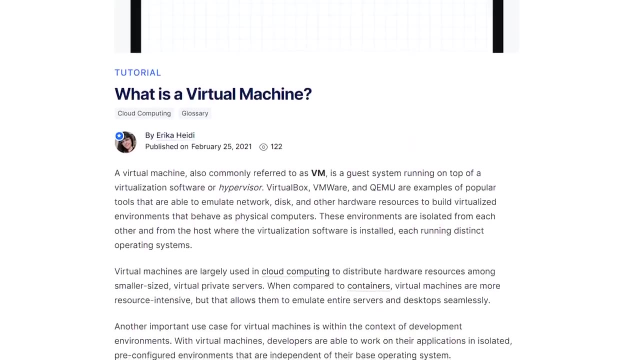 Gatekeeping aside. So here are some things you can do or implement into your life to mitigate the invasiveness of Windows if you're still dependent on it. First, use virtual machines. We've covered using virtual machines for improving privacy and security in Go Incognito. 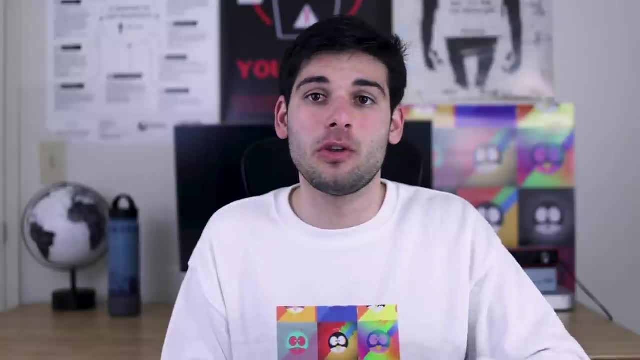 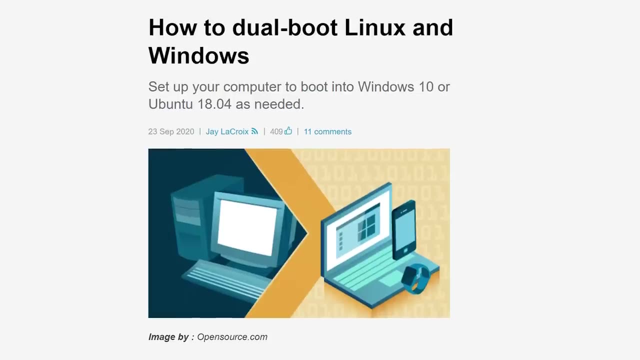 our course, and it stands true for this video as well. You can use Linux as a guest OS for your Windows computer, or you can fully migrate to Linux and use Windows inside a virtual machine. Second, you can dual boot Linux and Windows on the same system. 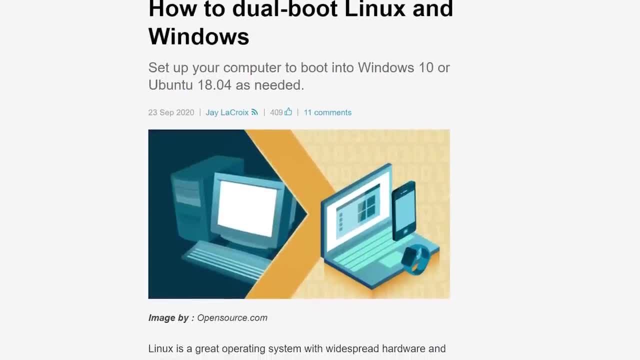 So if you have any questions, feel free to leave them in the comments below. Ideally on two separate hard drives, but you can do it on the same drive as well. This gives you a lot of compartmentalization while still letting you boot into Windows. 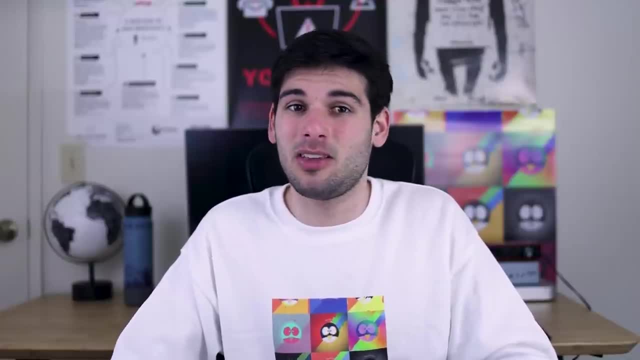 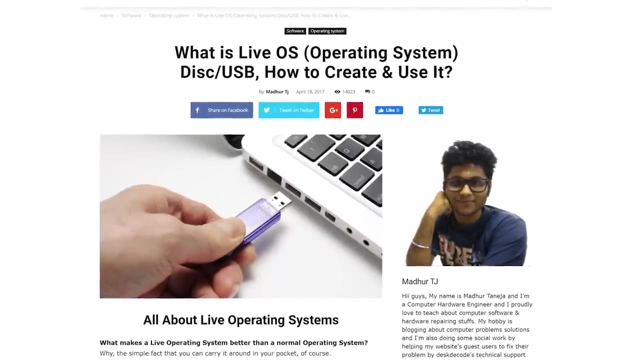 for certain things. Maybe Linux is used for everything except gaming, and that's the only data Microsoft gets about you. It's a pretty good solution to have. Third, there are live operating systems. These can be any generic Linux-istro like the Ubuntu Live OS, or it can be something. 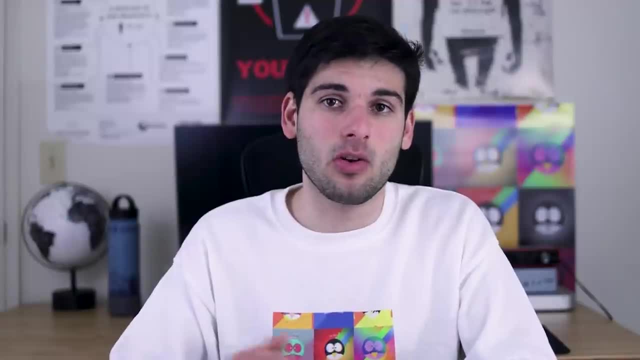 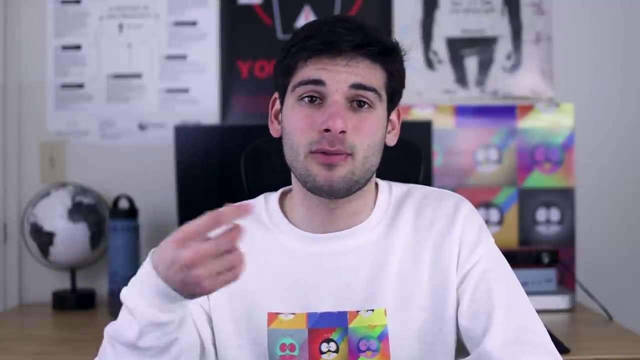 more hardcore, like Tails. The point stands: If you are stuck on Windows, don't want VMs and don't want to dual boot, but still need a safe place where you have peace of mind, you can always keep a nice flash drive that. 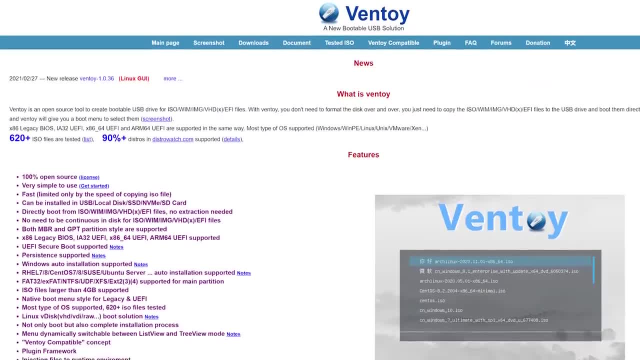 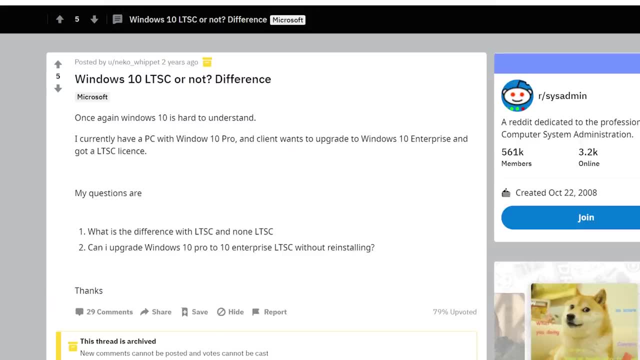 lets you access an OS that you can put a lot more faith in, And you can even use things like Ventoy Linux to install more than one operating system on a single drive. Fourth, there are actually variations of Windows, like Windows LTSC, that disable some of the 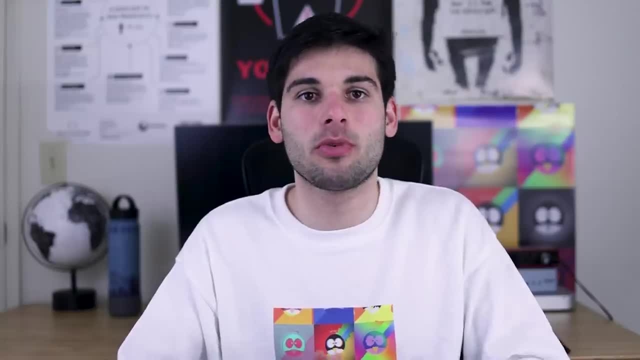 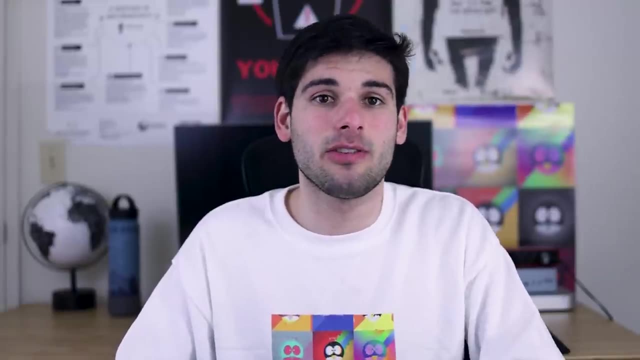 telemetry collection and don't send as many feature updates while still providing security updates, which is very important. These are not easy to come by, at least legally, and are not recommendations I can make to a lot of people, But just be aware that this is an option. 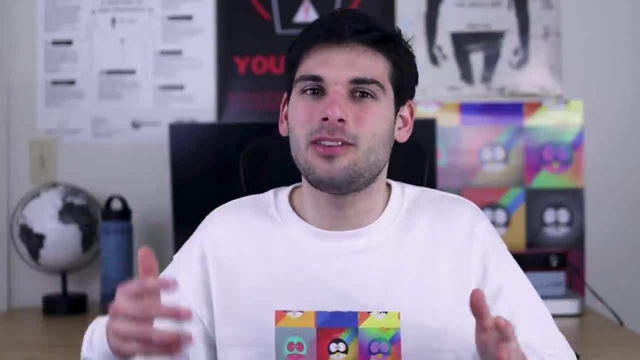 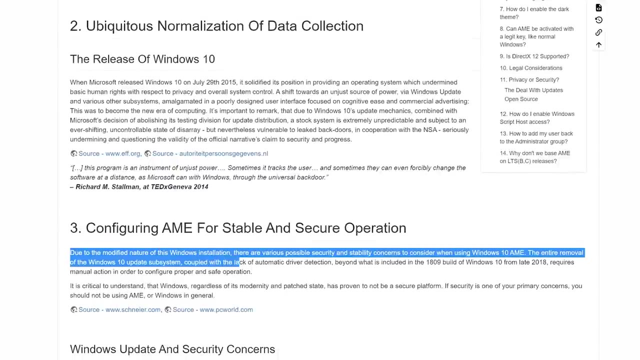 As for things like Windows AME, just don't Unless you have a good reason, But for most people don't. They don't easily get security updates and they publicly advertise that they are a privacy-only security-second tool, which is something we discourage, as security and privacy are two. 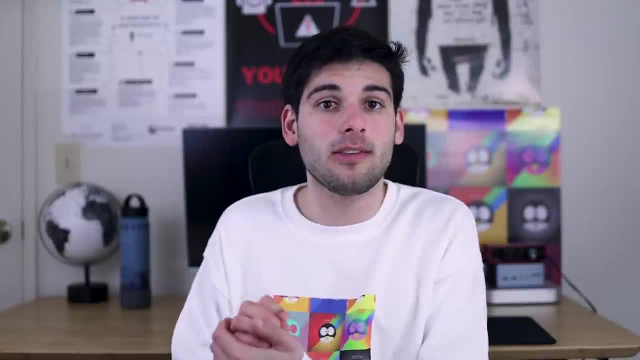 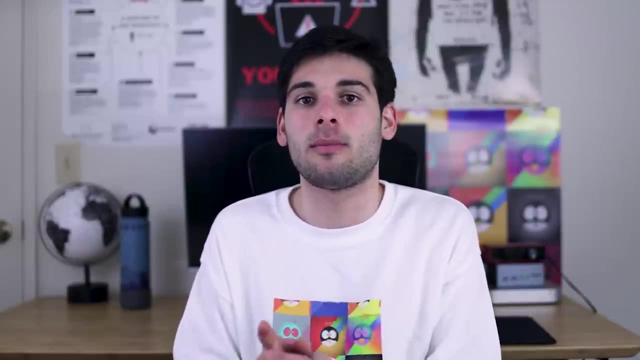 important sides of the same coin. I encourage people to stick to the official OS when you can and manually apply the patches if you choose to go this direction. I strongly discourage the use of Windows AME unless you have a very good reason for using it. 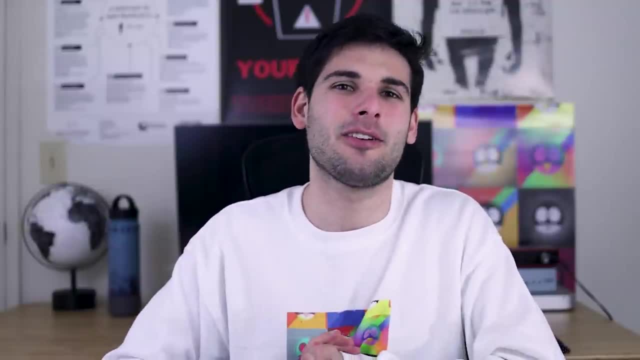 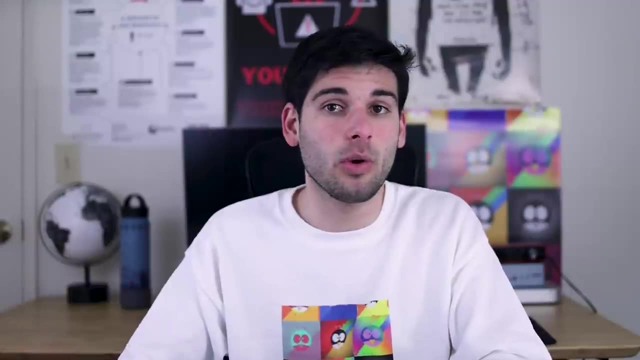 And that everybody is how you make Windows as private and secure as we can. It's important to emphasize that improvements are improvements and you shouldn't listen to those annoying people who immediately dismiss Windows without understanding why a user may be dependent on it. okay, 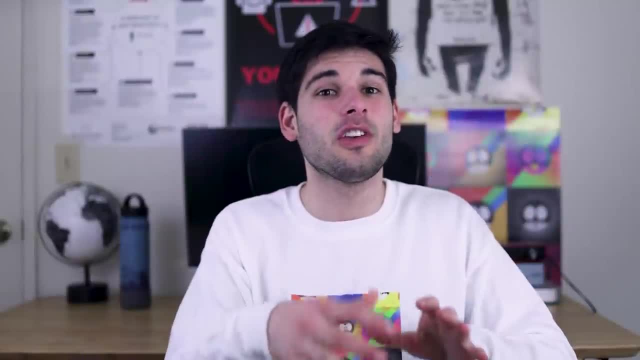 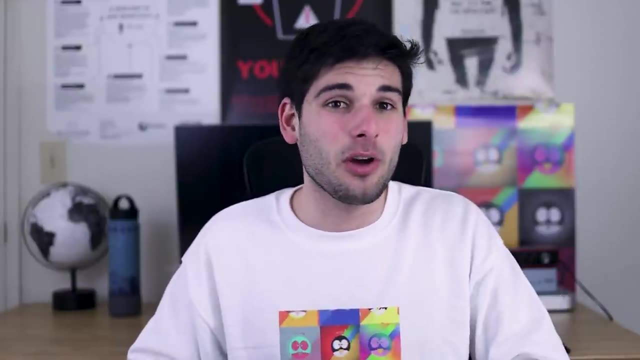 We get you. We're here for you, We're listening. The OS you choose is your decision and we will help you as much as we can to get you to where you need to go, while still maintaining your configuration. If you liked this video, we made an iOS and Android version of it so you can bring all. 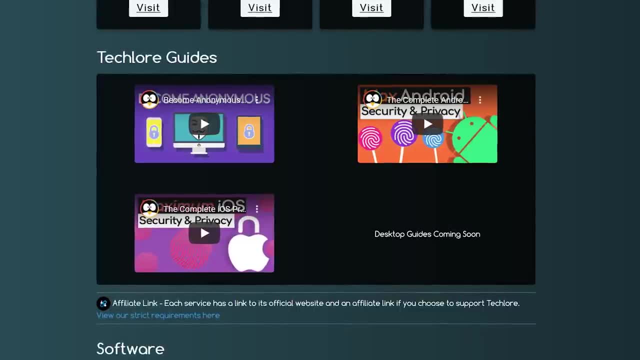 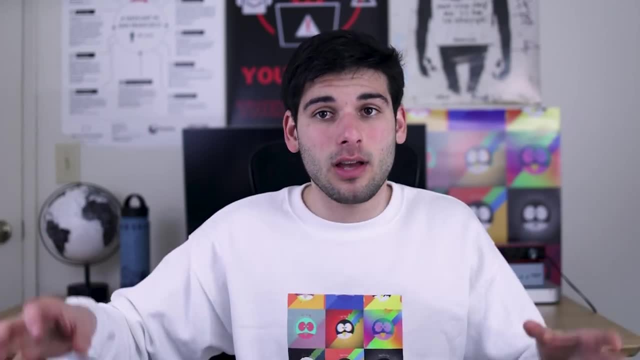 of your devices to Mac Safety, And we even made an all-encompassing Become Anonymous guide for broader advice applicable to everything. All of these use the similar 3-Zone system. Aside from this, if you really want to dive into the world of privacy, our Go Incognito. 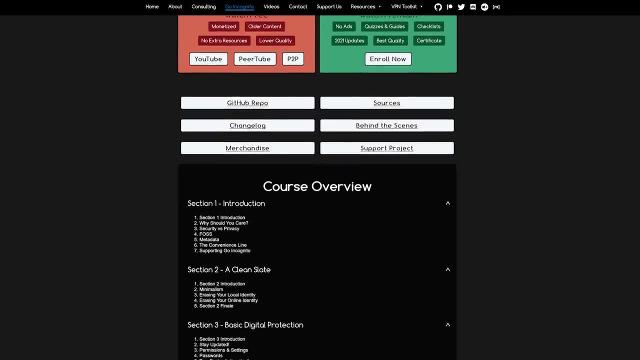 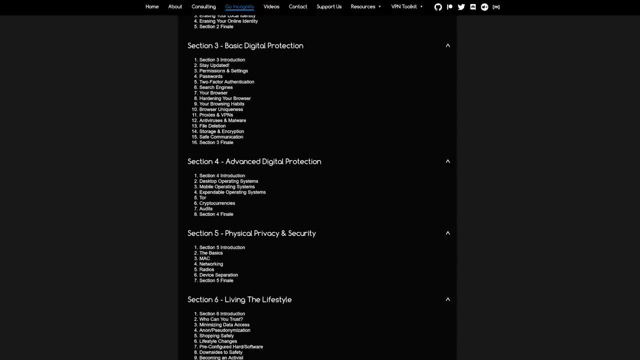 course is a phenomenal way to not only learn the ropes but finish feeling confident in your ability to protect yourself online. It's like four hours of just in-depth knowledge, so it's very well laid out. You're going to learn a lot if you take that. 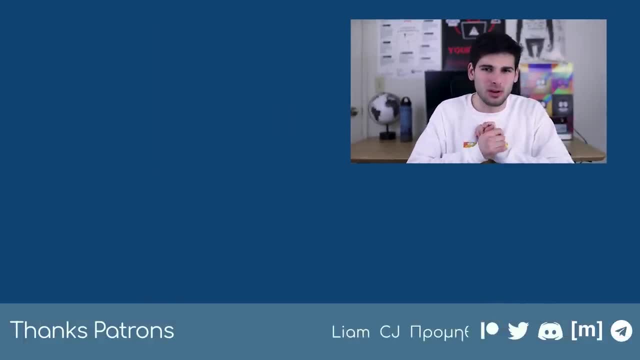 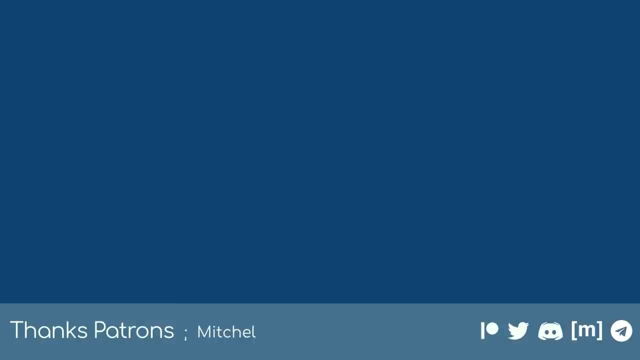 Don't forget to like and subscribe. and a massive thanks to our supporters who believe in our mission and spreading privacy and security to the masses. I want to thank you for watching and I'll see you next time on Techplore.